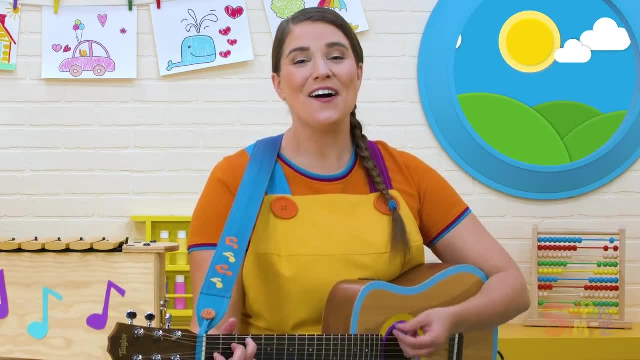 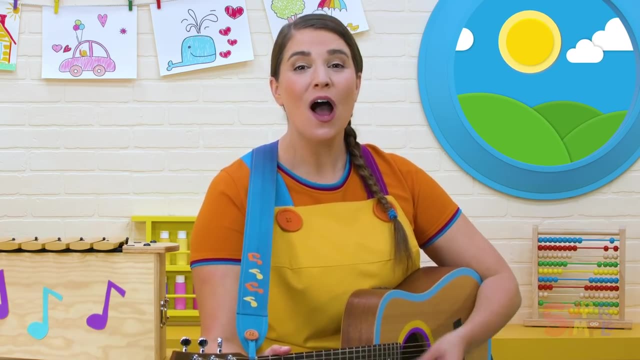 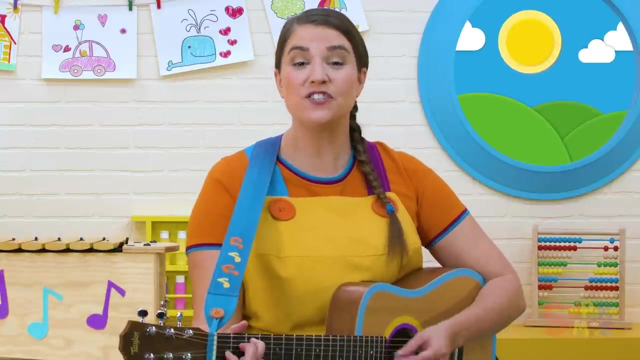 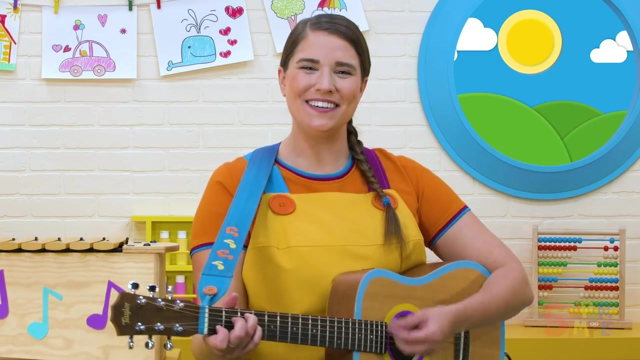 Here we go. Hello, hello, What's your name? Hello, Hello, What's your name? My name is Caitie. What's your name? Can you shout it out? nice and loud: Nice to meet you, Let's be friends. 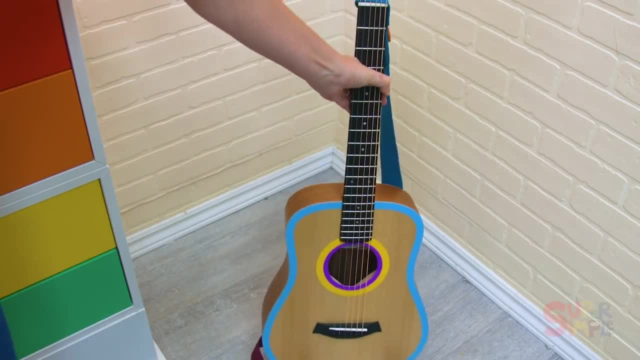 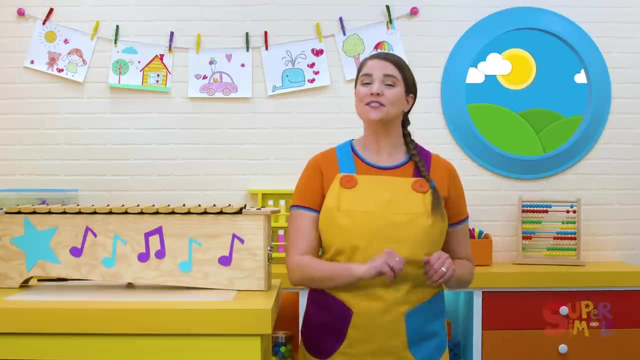 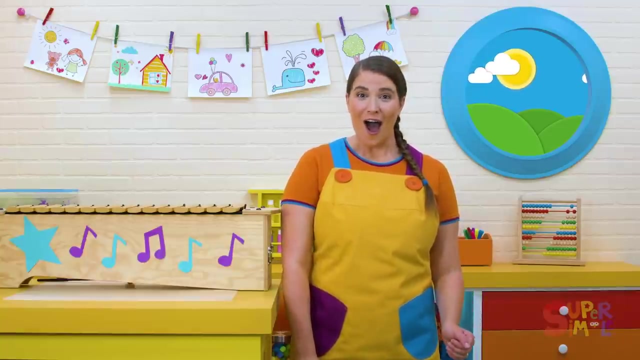 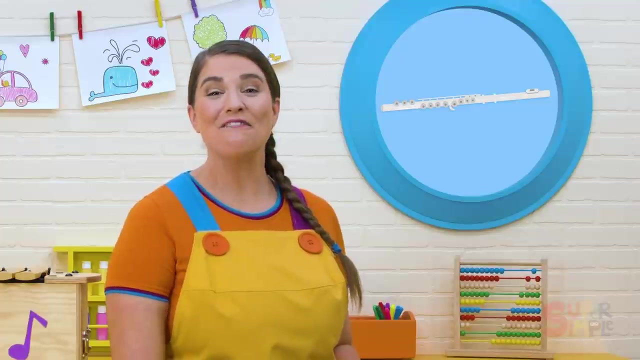 Hooray, That song sounds a little different played on guitar, doesn't it? Each musical instrument has their own special sound. Hello Yo, hello, Wow. What musical instrument was that? Oh, It's a flute. A flute is played like this: 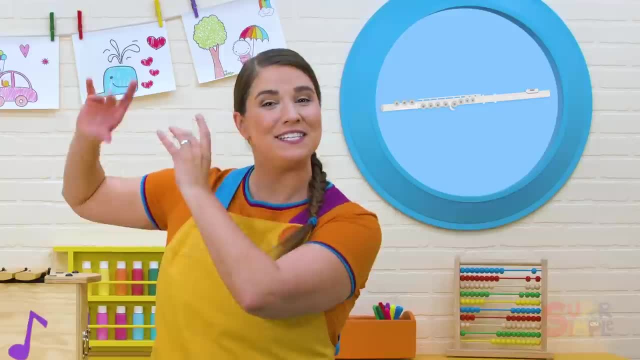 We use our mouths to blow air over a hole to make the sound. Let's pretend to play the flute together, everyone. You want to hear a different flute? You want to hear a different flute? Do you want to play one of them? 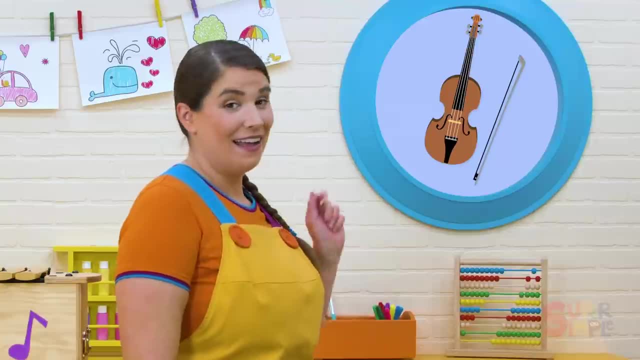 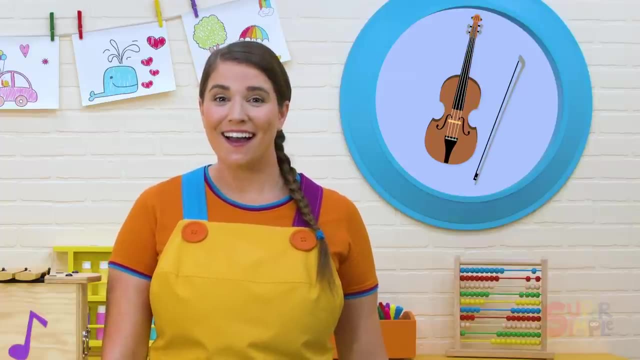 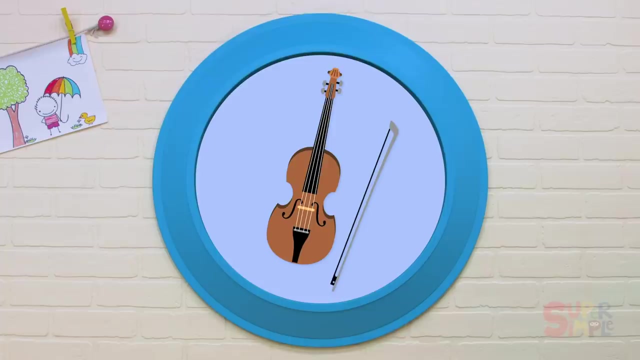 Nice flute playing. This is a violin. Let's hear what it sounds like. Oh, I like the violin. A violin is played with a bow. The bow moves across the strings to make the sound. Let's pretend to play the violin. 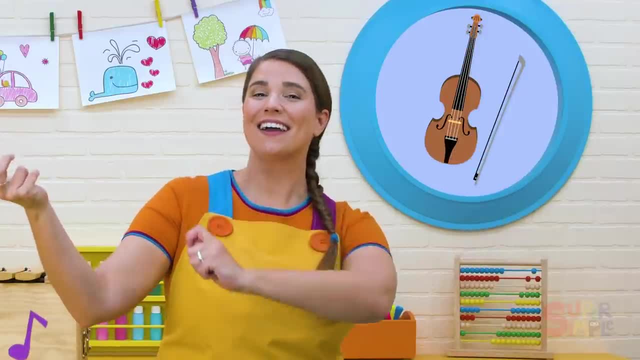 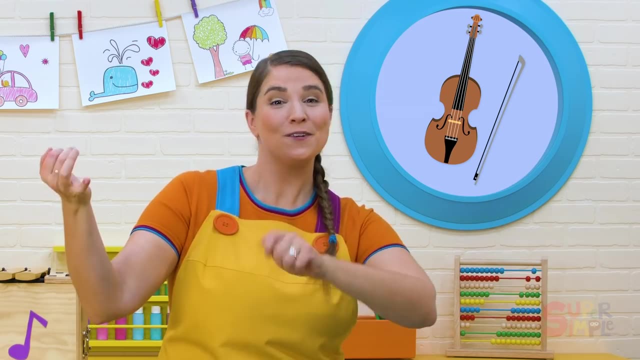 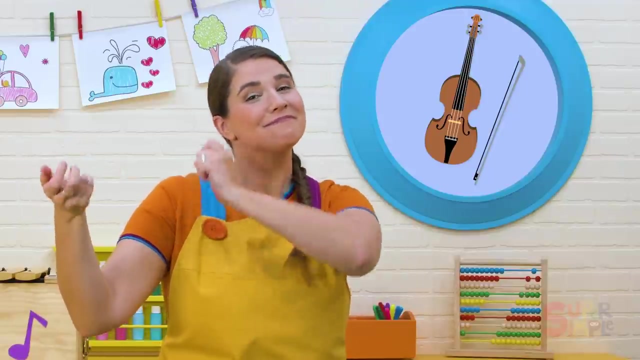 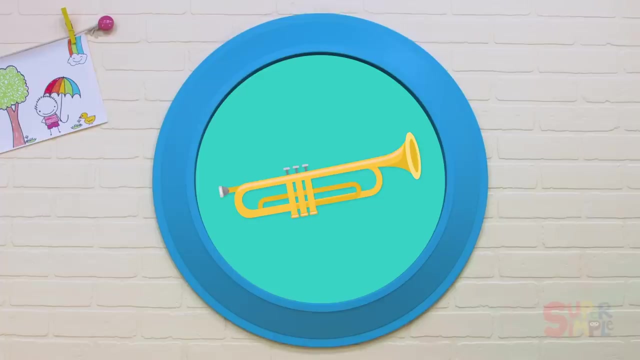 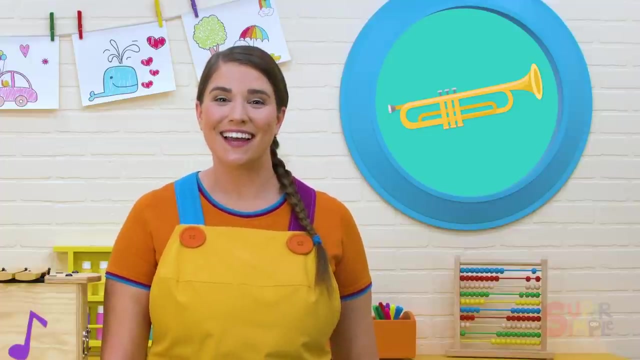 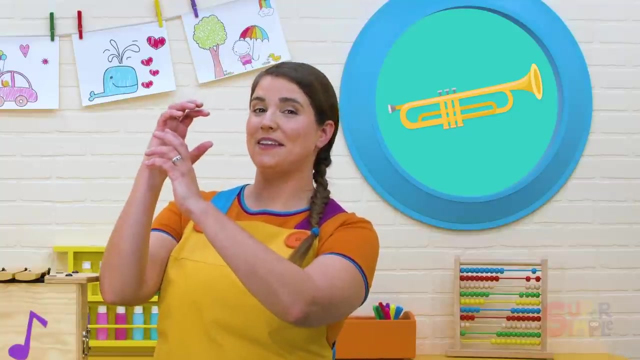 Are your bows ready? Here we go. Excellent violin playing. Ah, it's a trumpet. I like this sound a trumpet makes. Let's listen. Oh, it's a neat sound To play the trumpet. we use our mouths to make a buzzing sound. 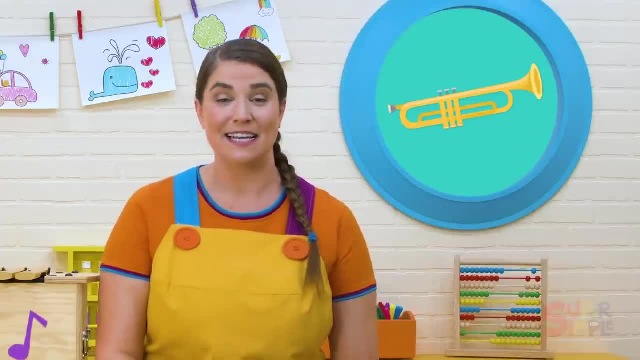 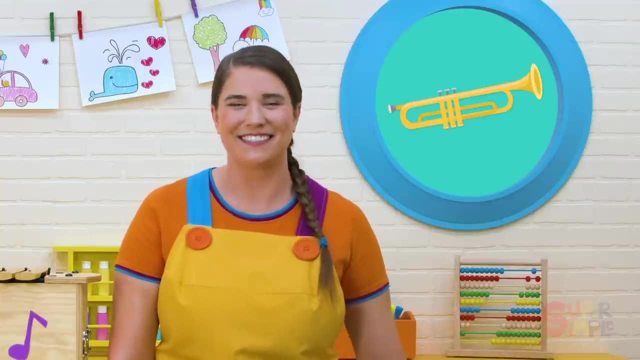 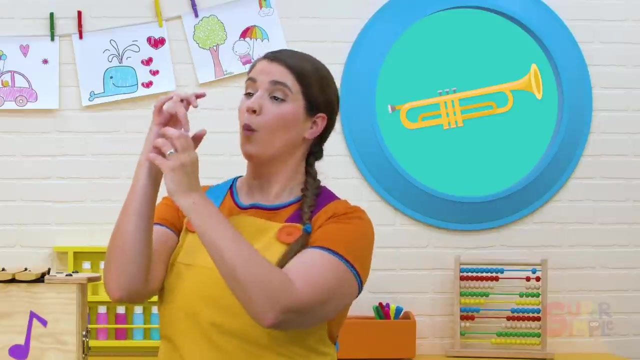 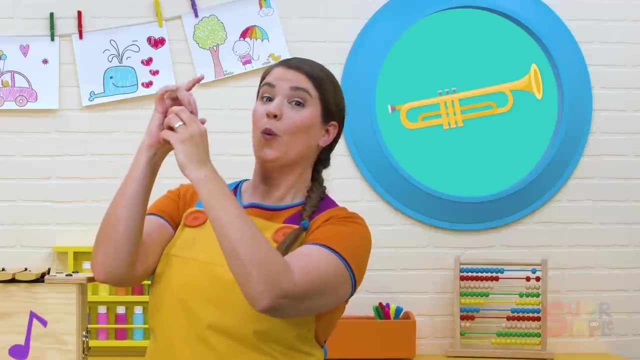 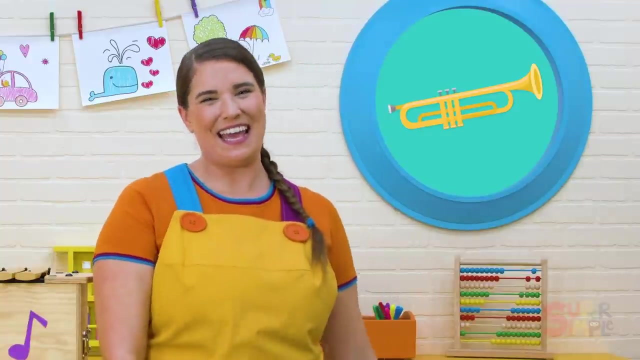 and blow into the mouthpiece, Kind of like a trumpet, Kind of like. this Sounds pretty silly without the trumpet, doesn't it? Well, let's pretend to play the trumpet all together: Great trumpet playing. Let's hear what it sounds like. 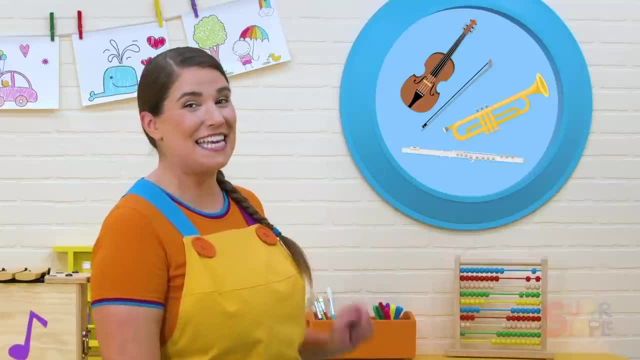 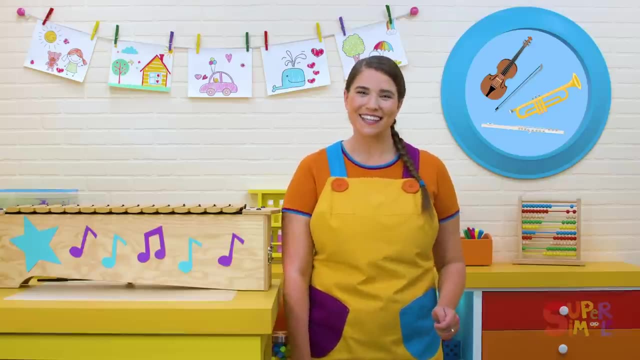 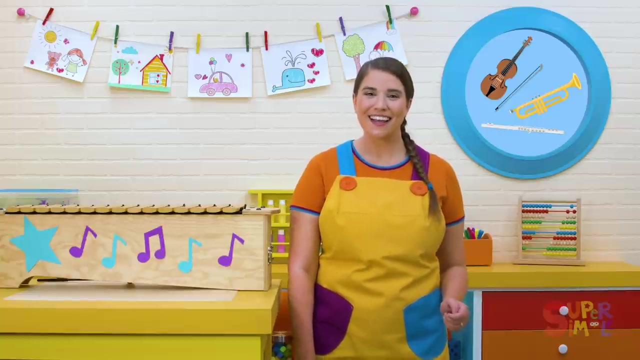 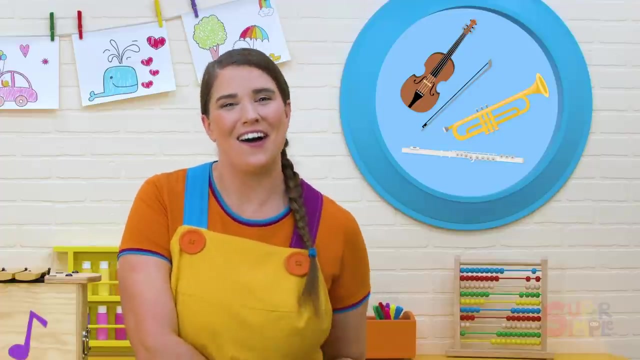 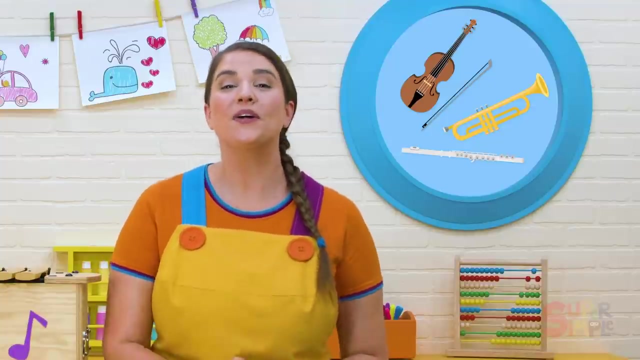 when these three instruments play all together. Ooh, such beautiful sounds. Okay, Let's see if we can remember to play the trumpet. Let's see if we can remember all the instruments we heard. with a little game, We'll listen to one of the three instruments. 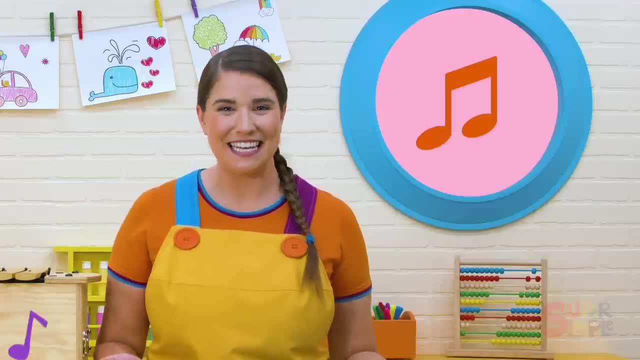 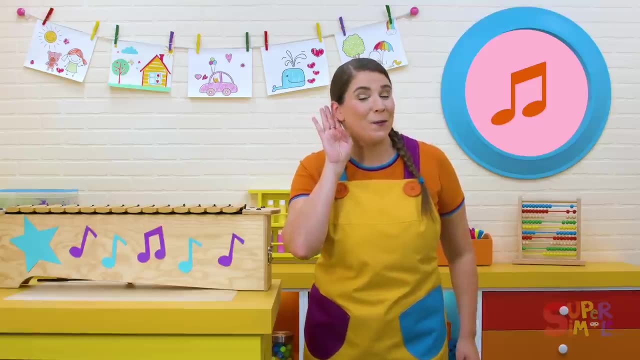 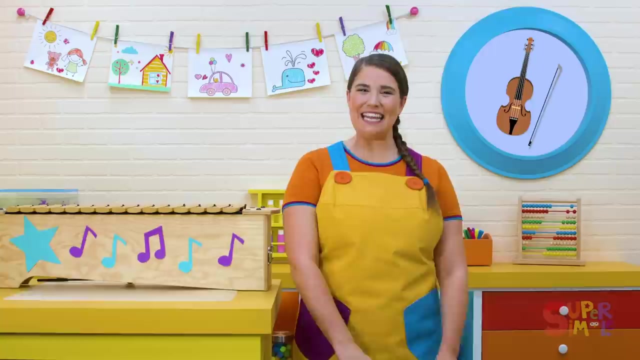 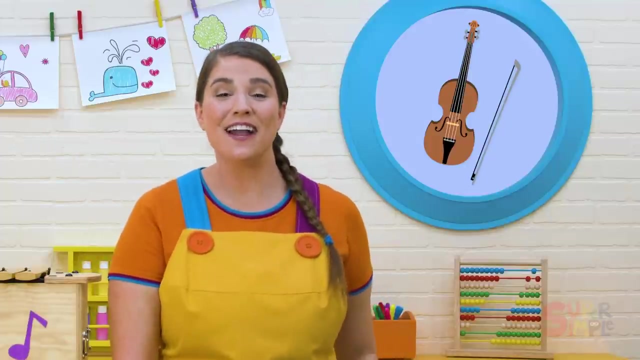 We'll try and guess which one it is. Are you ready? Okay, Let's listen. Ooh, do you remember what instrument makes that sound? I think I know The violin. That's it. Let's try another one. Listen closely. 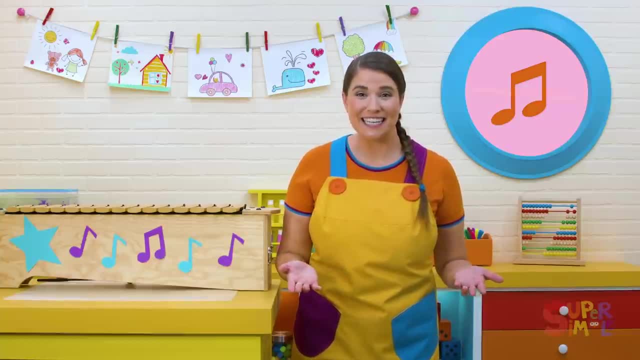 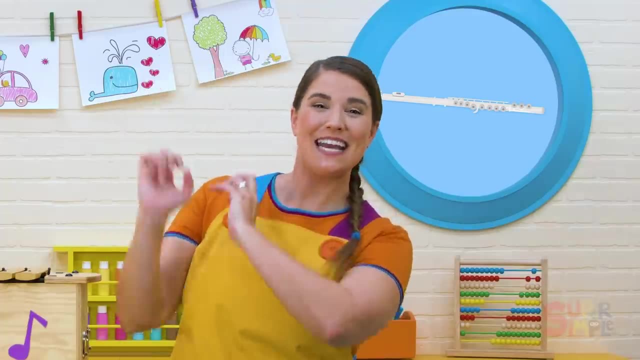 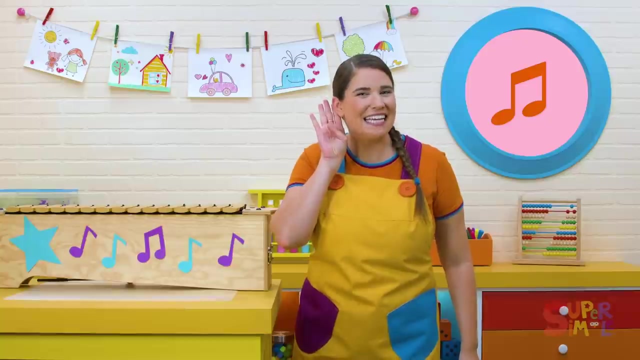 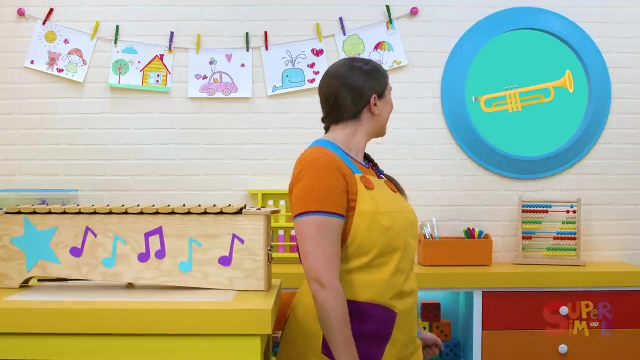 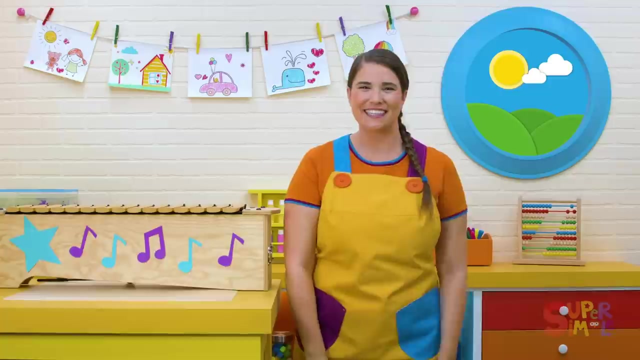 Do you remember that sound? Any guesses? The flute, Nice job, One more, Let's listen. What's that one? The trumpet, Ooh Yeah, great job everybody. Let's pretend to play those three instruments and more with a song. 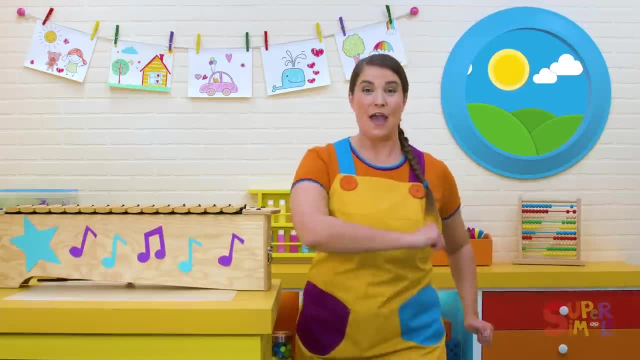 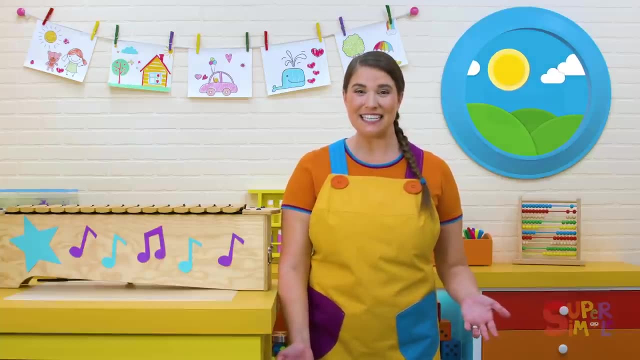 We'll sing when the band comes marching in, and we'll try some new instruments too. I hear one now. Do you know what instrument this is? Ooh, that sounds good. do you know what instrument this is? It's a drum. 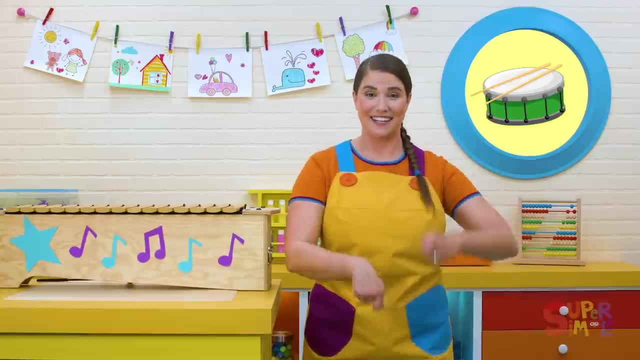 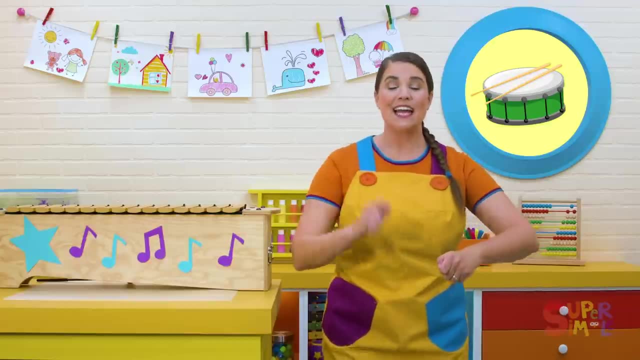 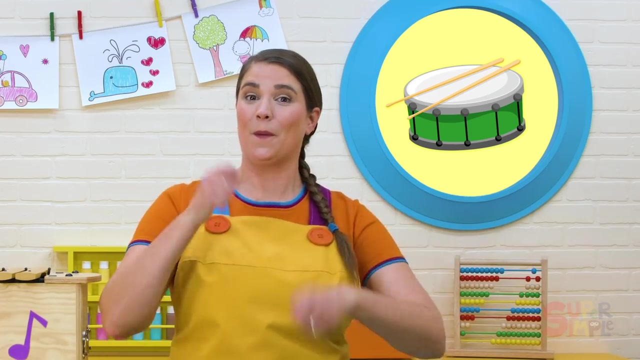 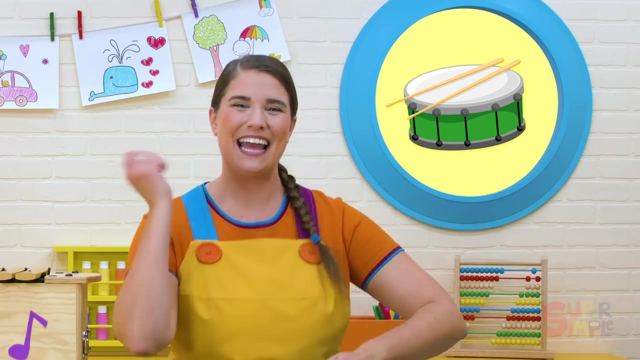 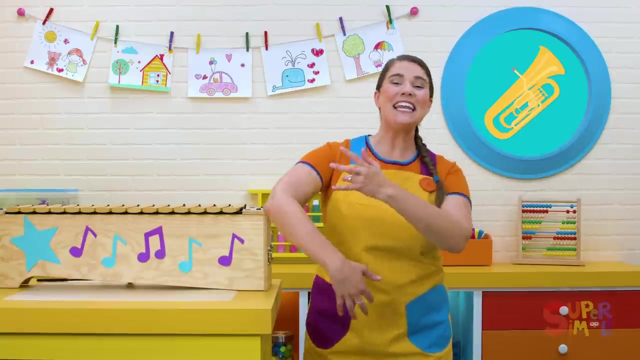 Let's pretend to play the drum together and march. Here we go. Oh, when the drum comes marching in. Oh, when the drum comes marching in, It goes. When the drum comes marching in, That's a tuba. Oh, when the tuba comes marching in. Oh, when the tuba comes marching in, It goes. 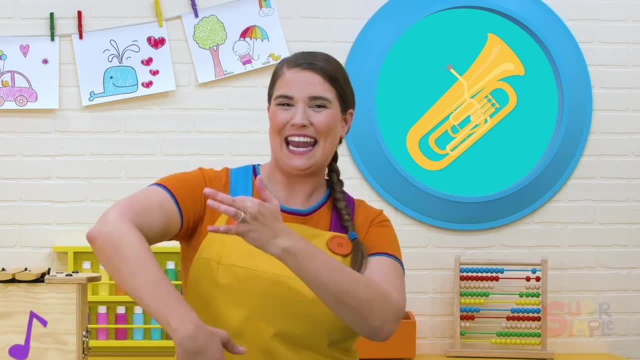 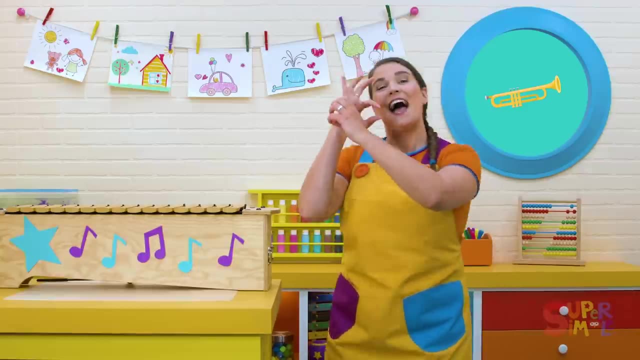 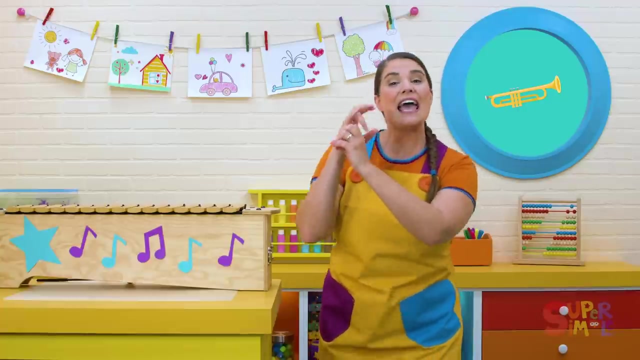 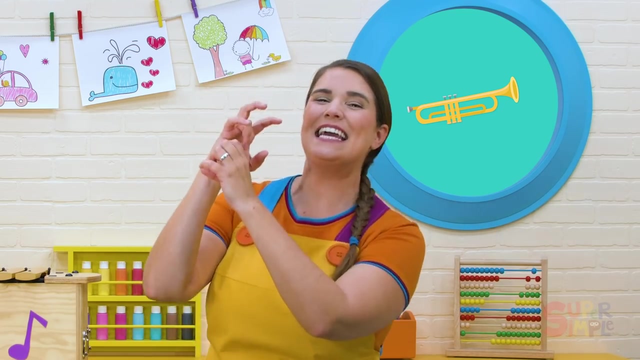 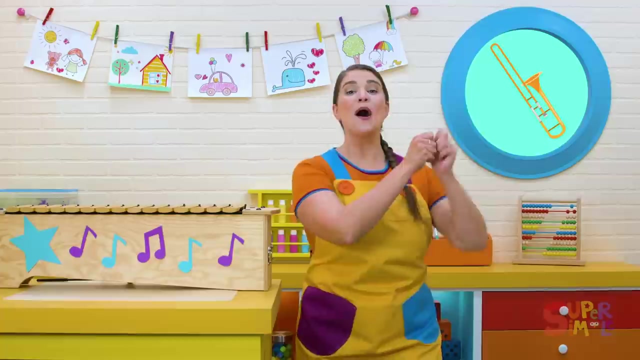 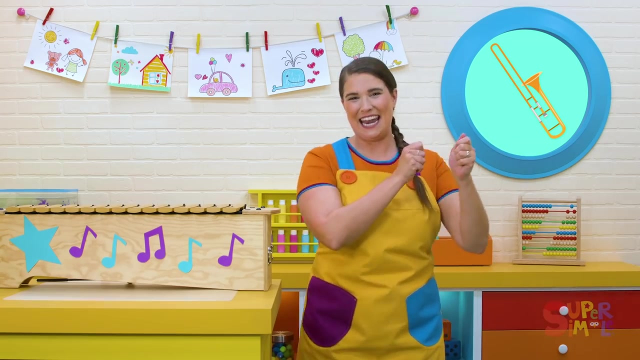 When the tuba comes marching in The trumpet, Oh, when the trumpet comes marching in. Oh, when the trumpet comes marching in, It goes. When the trumpet comes marching in, That's a trombone. Oh, when the trombone comes marching in, Oh, when the trombone comes marching in. 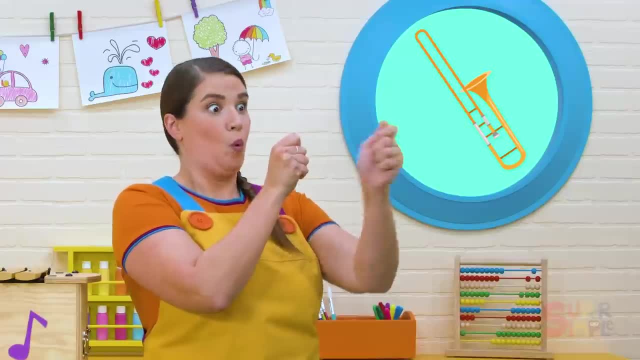 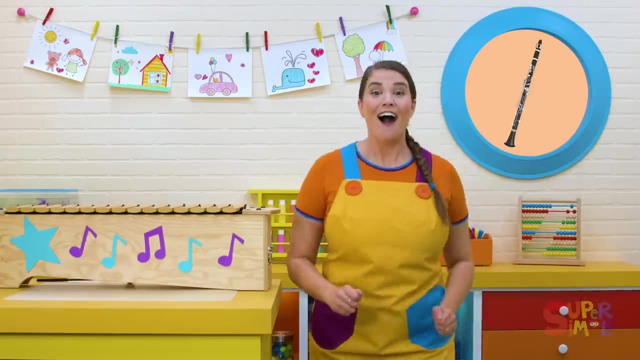 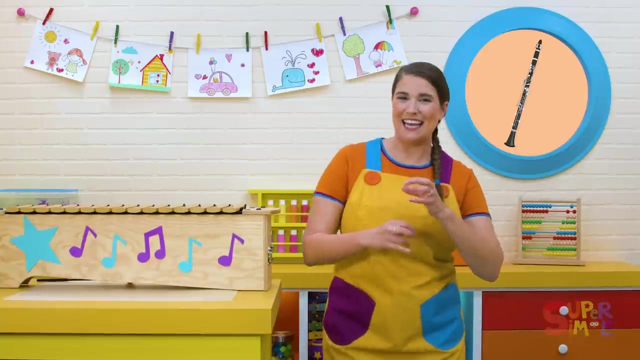 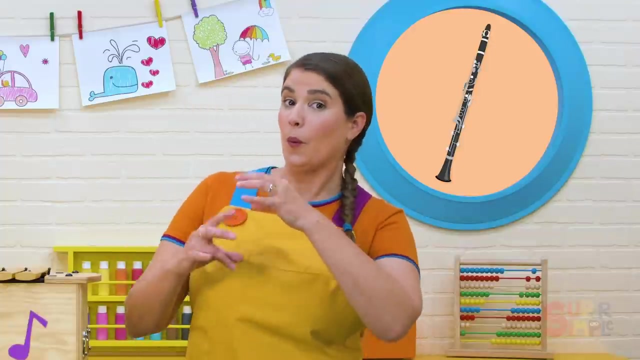 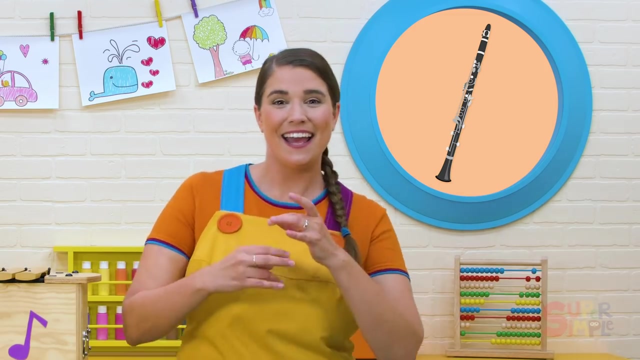 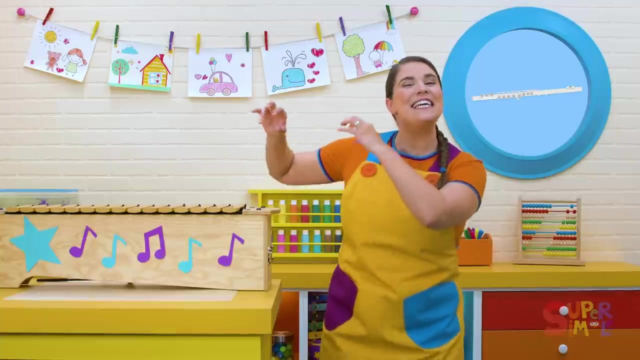 It goes. trombone comes marching in A clarinet. Oh when the clarinet comes marching in. Oh, when the clarinet comes marching in. It goes When the clarinet comes marching in. We know that one. The flute. Oh when the flute comes marching in. Oh, when the flute comes marching in. 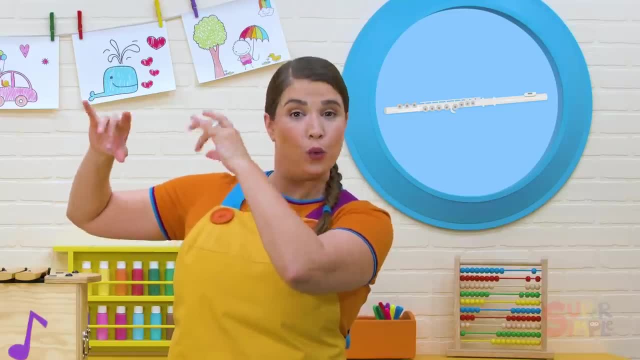 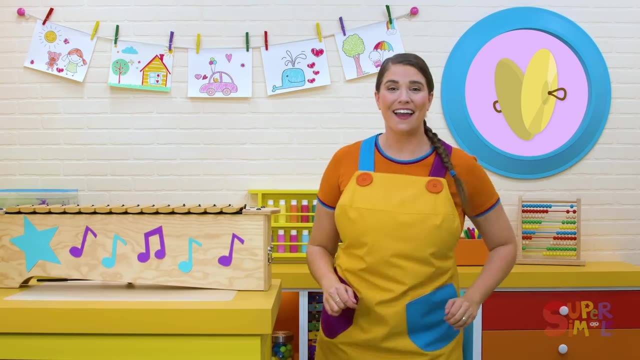 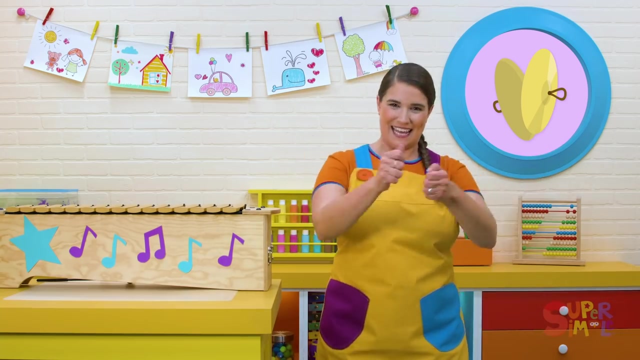 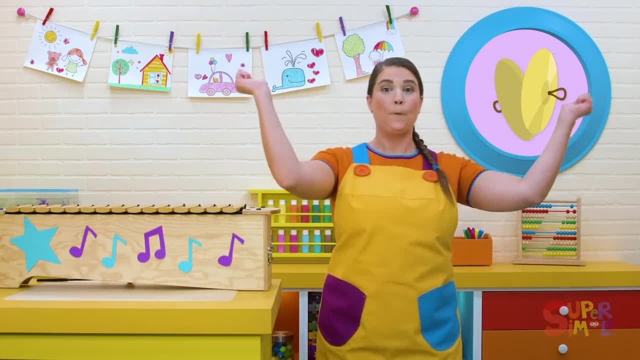 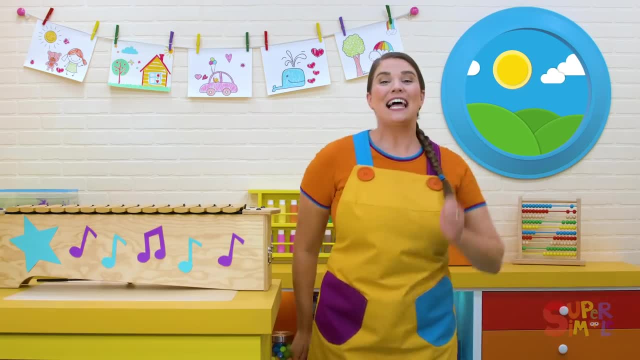 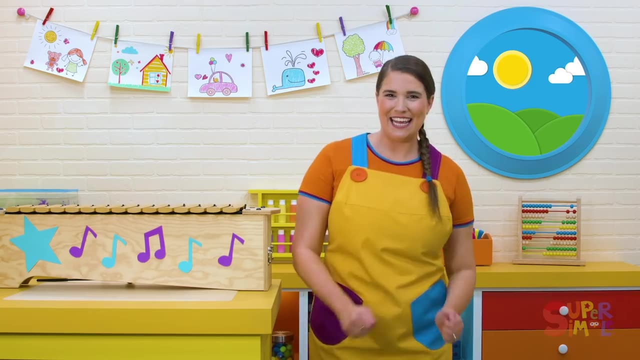 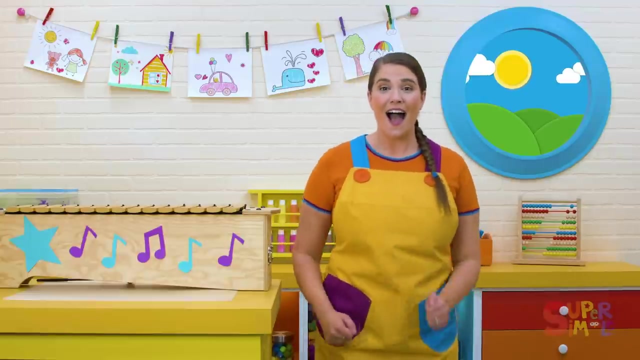 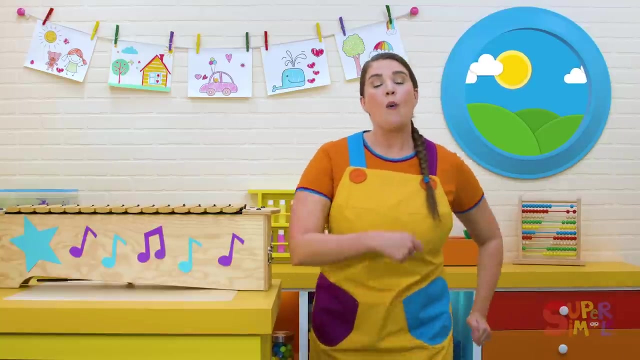 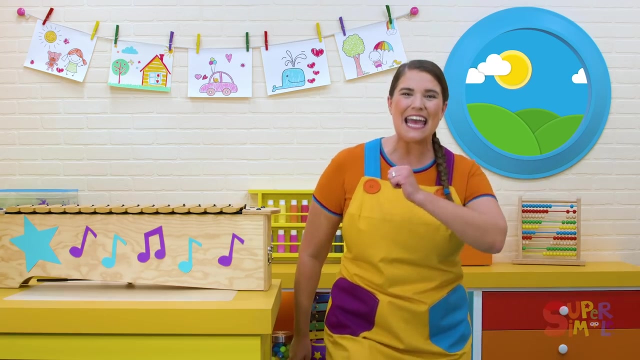 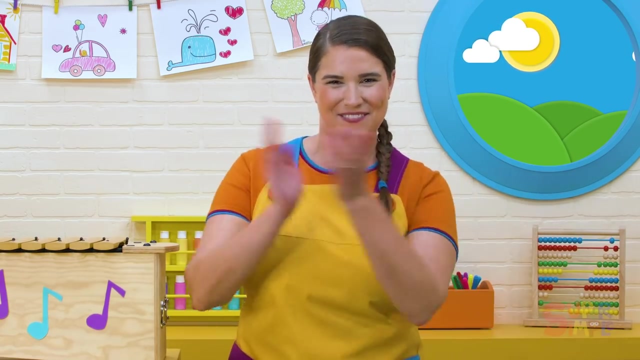 marching in, Let's play all together. Oh, when the band comes marching in. Oh, when the band comes marching in, It goes. When the band comes marching in. oh, when the band comes marching in, So great, Give yourselves a big clap. 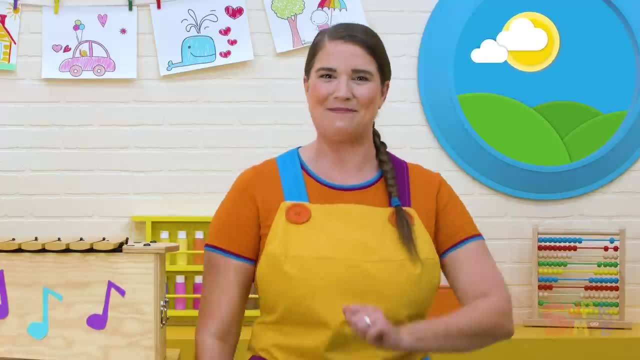 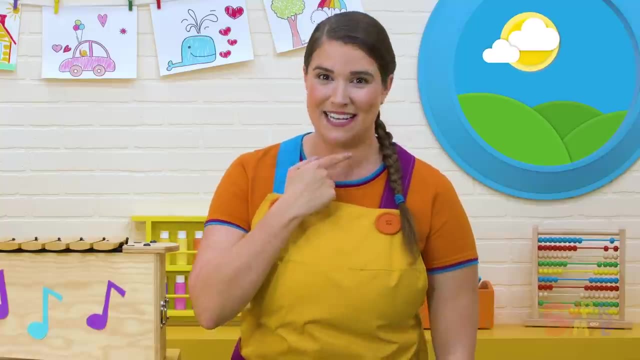 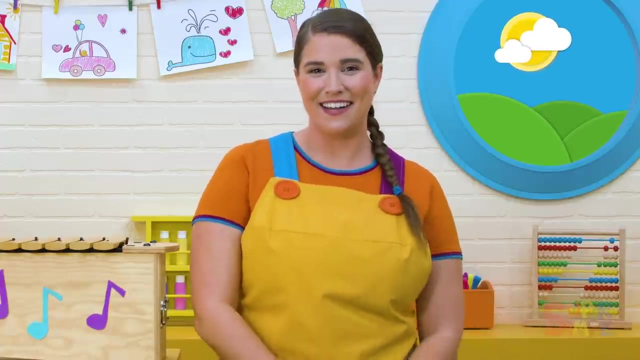 There are so many amazing instruments in that marching band. Did you hear the trumpet And the flute? Our voice is an amazing instrument too. We use it to sing la, la, la. just like we sang the song, We can sing low, low. 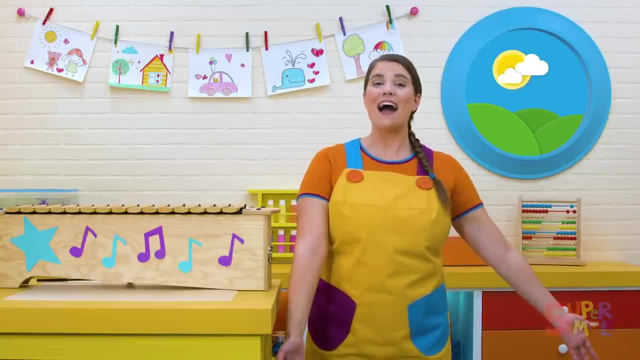 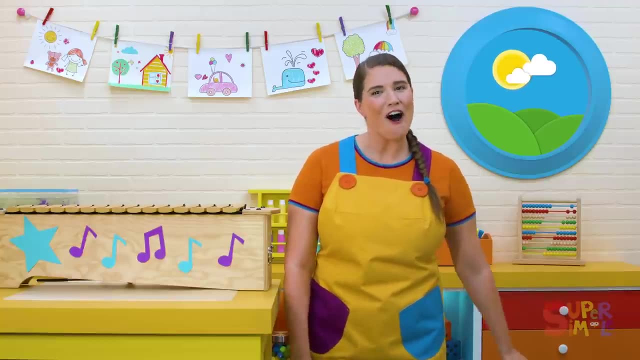 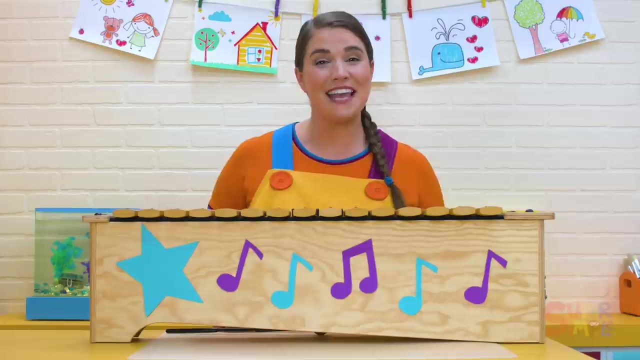 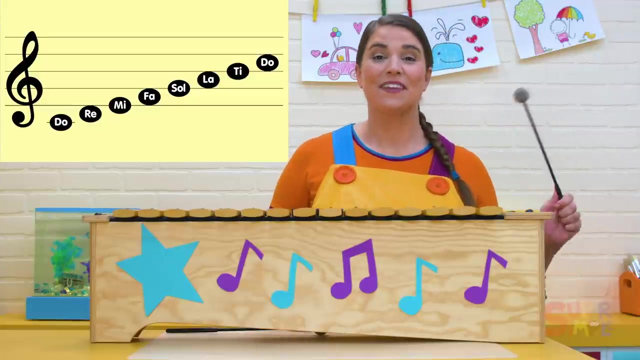 And we can sing high, high And all the notes in between. Let's practice an instrument we have all the time: our voice. We can use our voice to sing a scale. A scale is a set of musical notes. Here's a scale. 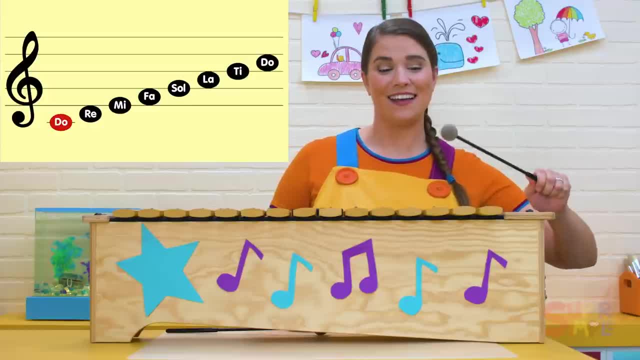 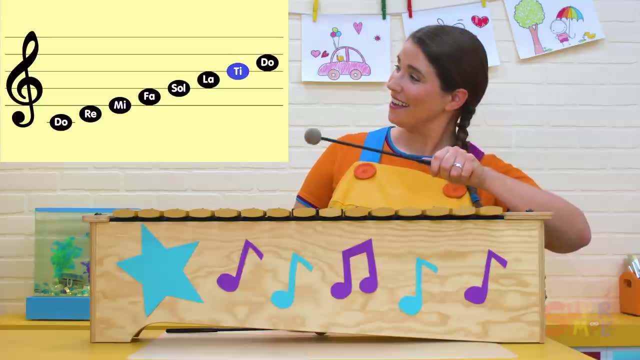 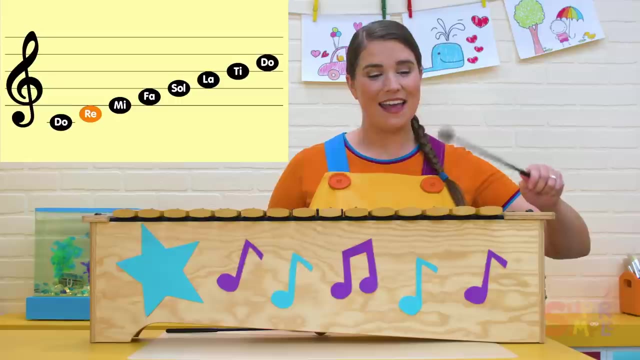 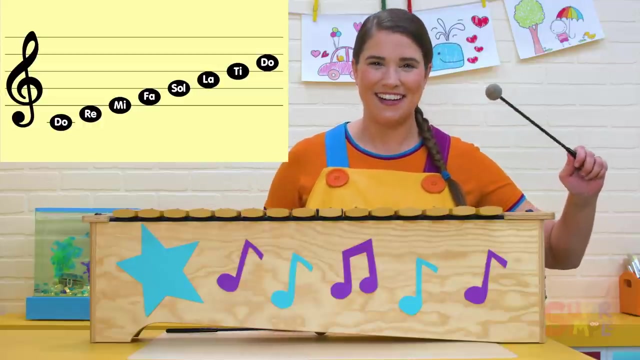 I'll play the notes on the xylophone. Each note has a name: Do re mi fa, so La ti do. Let's use our voice and we'll sing up the scale together. Here we go. 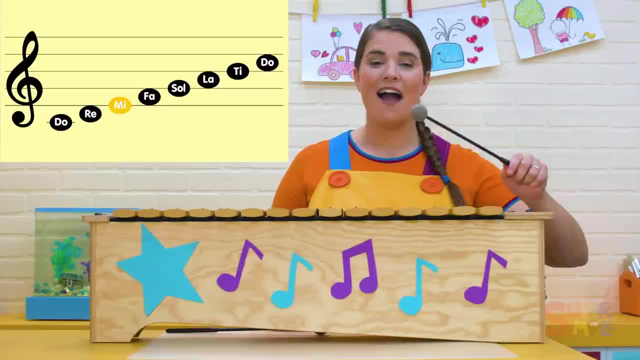 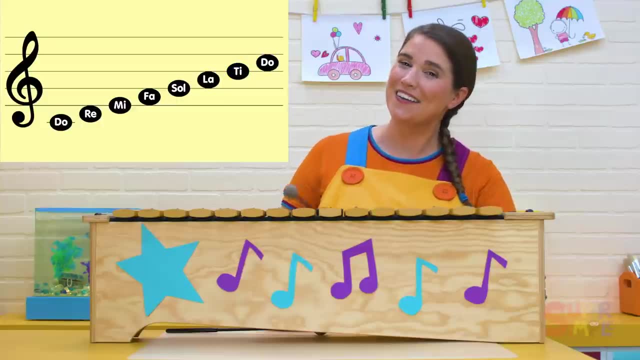 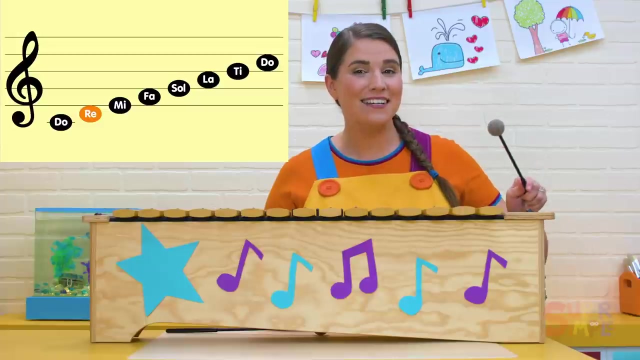 Do re mi fa so La ti do. Very nice. Now let's sing down the scale. Do ti la so Fa mi re do. Beautiful. Let's put those two together. 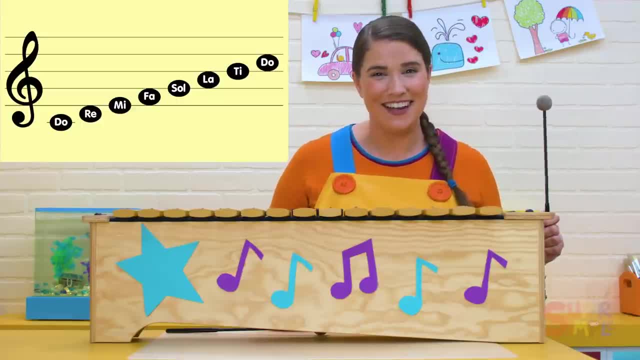 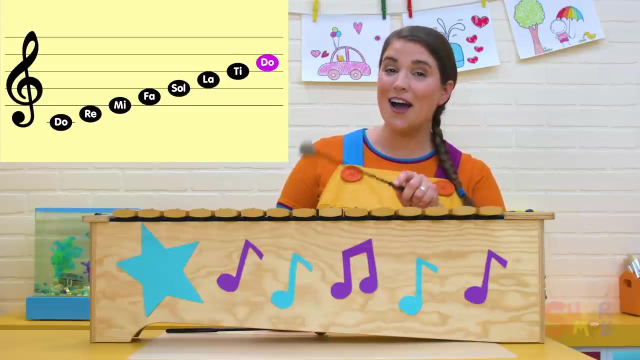 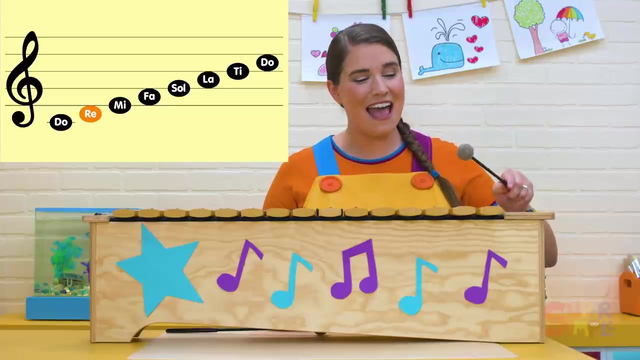 We'll sing up the scale, then back down. Are you ready, Here we go. Do re mi fa so La ti do. Do ti la so Fa mi re do. 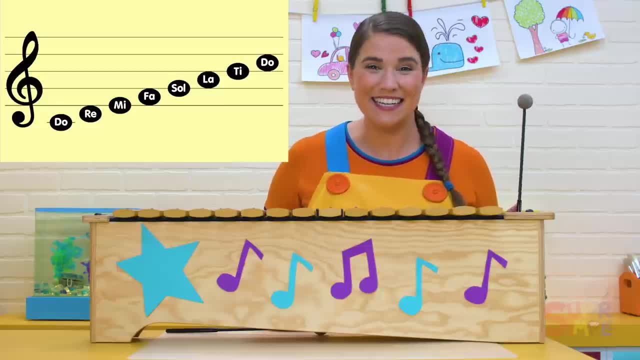 That's it, Shall we try going faster. Sing along with me: Do re mi fa so La ti do. Do ti la so Fa mi re do. Let's try going super fast. 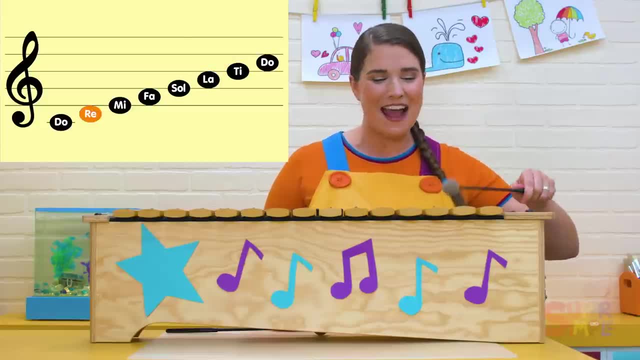 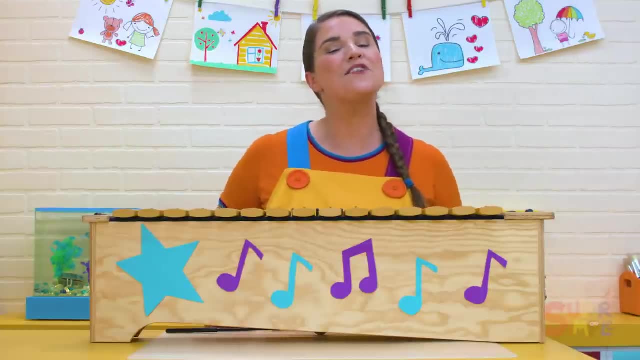 Do re mi fa so La ti do. Do ti la so Fa mi re do. Nice job, Beautiful singing everybody. We have a wonderful musical instrument right here: our voice. 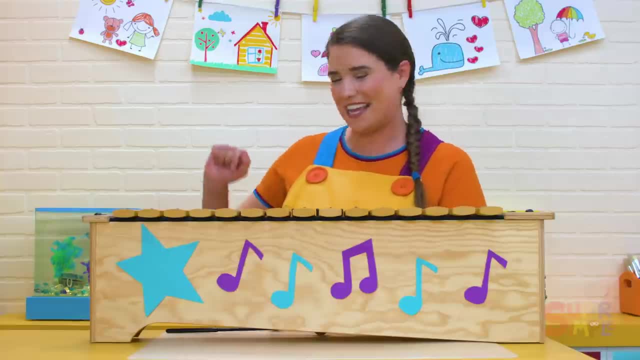 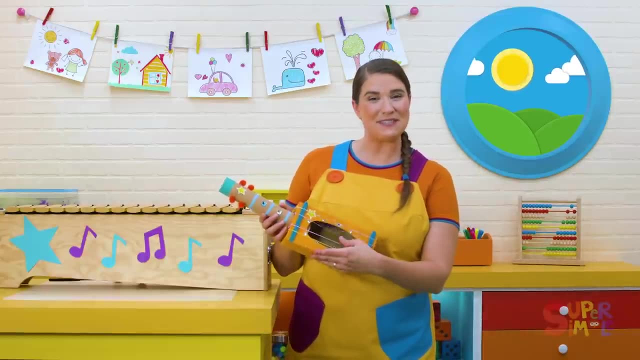 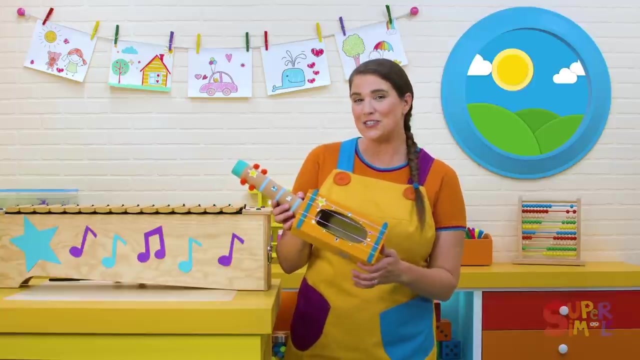 I have another wonderful musical instrument right here. Take a look at this. It's a craft I made. Do you know what instrument it's supposed to be? A guitar, yeah, just like the guitar we have in the classroom. I'll show you how you can make one like this at home. 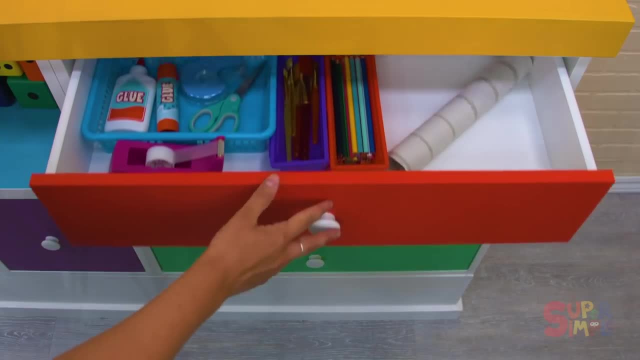 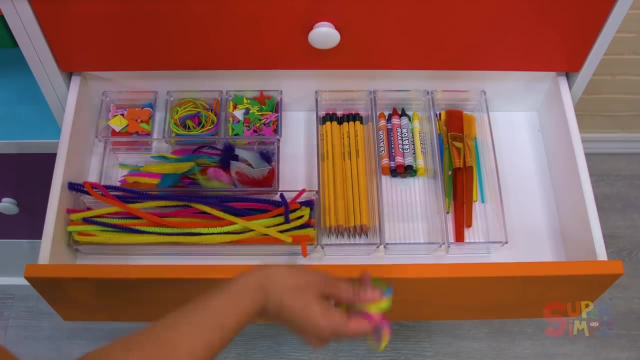 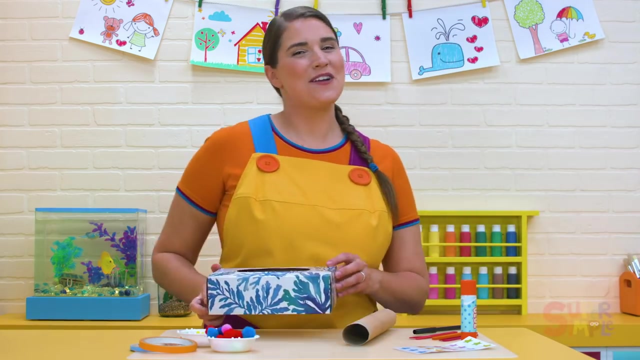 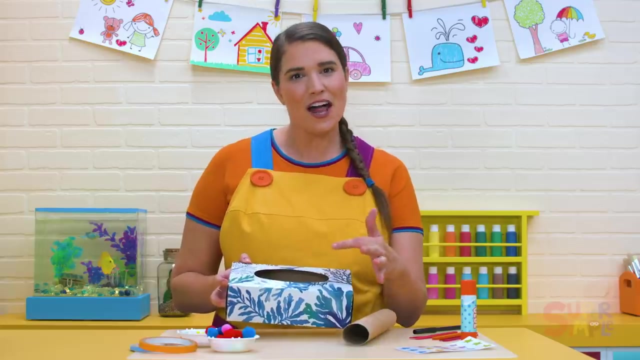 Let's gather the things we need. Some things we need for this craft are a long cardboard tube, elastic bands, a tissue box and a grownup. The tissue box is going to be the body of our guitar. The hole in the box is a lot like the holes that we see in a lot of guitars. 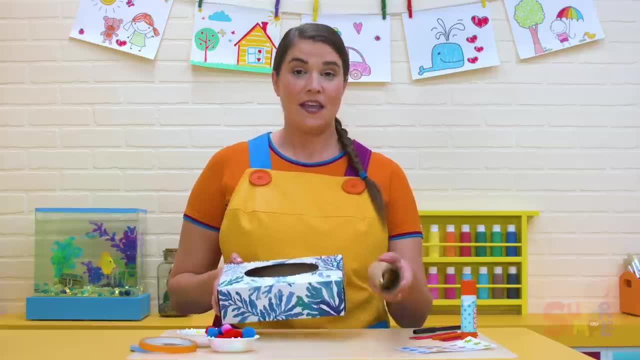 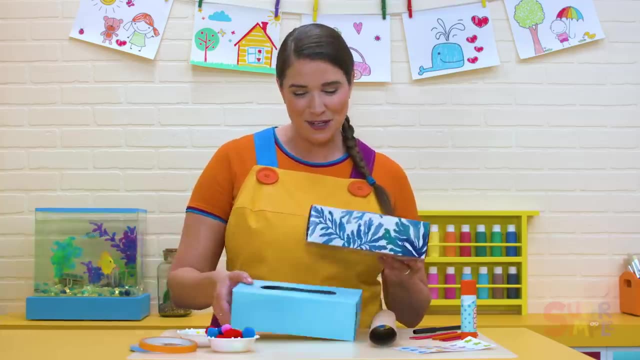 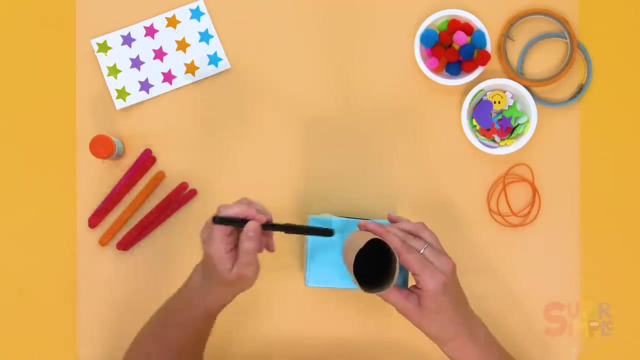 The cardboard tube is going to be the neck of our guitar. You can paint them both any color you like. I painted my tissue box my favorite color, blue. It's dry and all ready to go. We'll attach our cardboard tube by tracing the end of it onto one side. 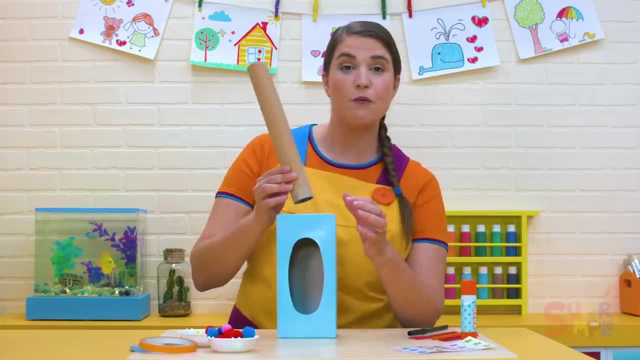 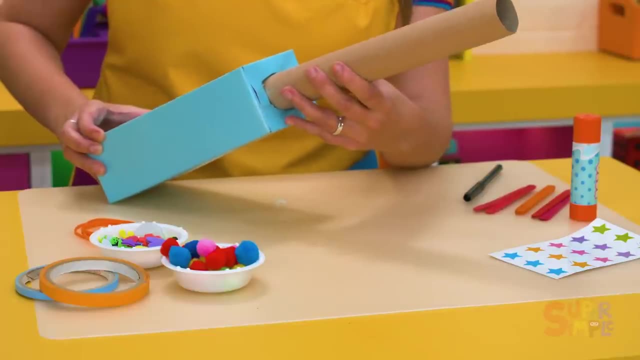 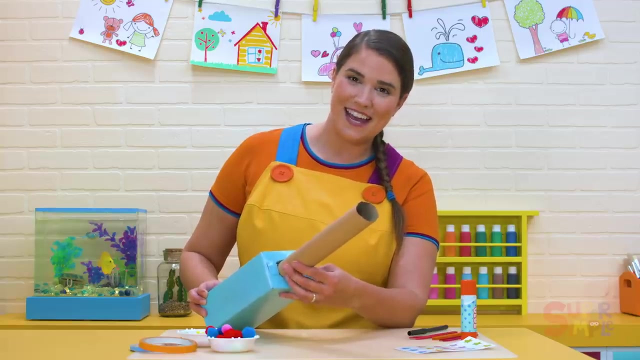 Then a grownup can help you carefully cut that out. like this: We're going to put the cardboard tube inside. It doesn't have to be perfect, because once the cardboard tube goes in, if it's a little bit smaller, it'll stay nice and snug in place. 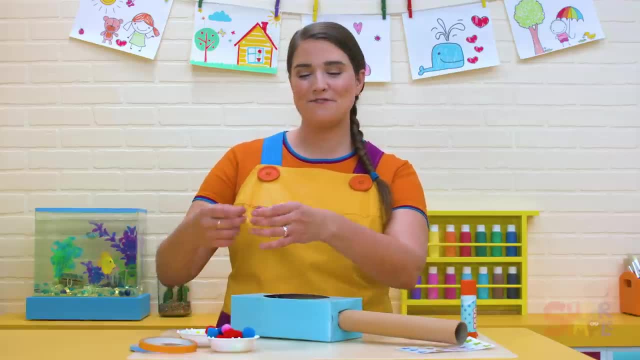 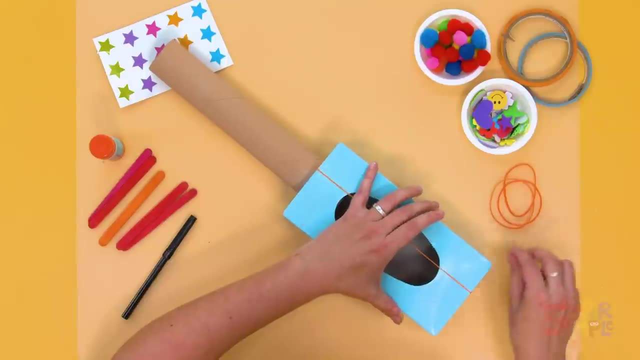 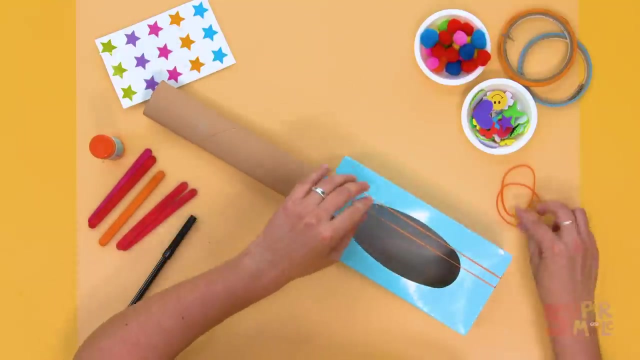 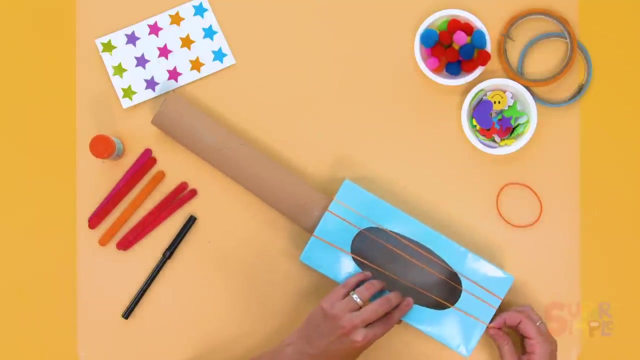 There. Now our guitar is ready for our strings. We're going to use elastic bands. I have some orange ones here. We're going to add four elastic bands: two on the top of the cardboard tube and two on the bottom. My guitar in the classroom has six strings, but this is a crafty guitar so it has four. 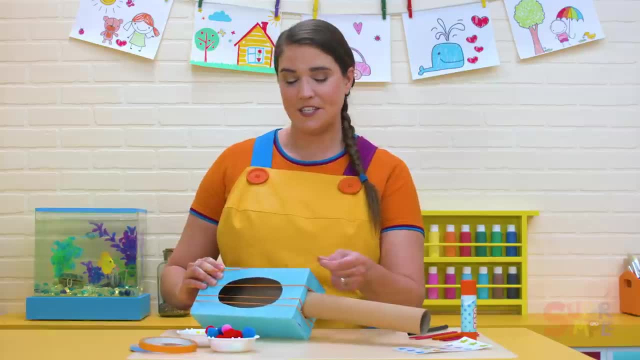 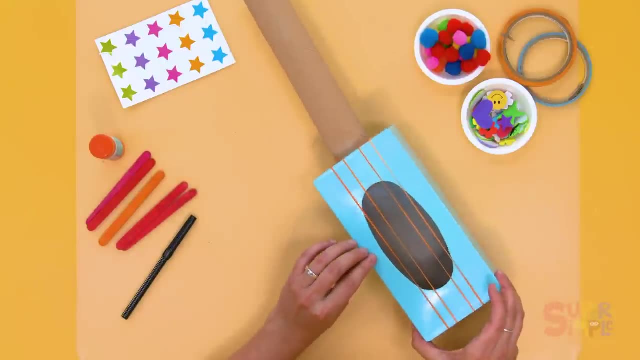 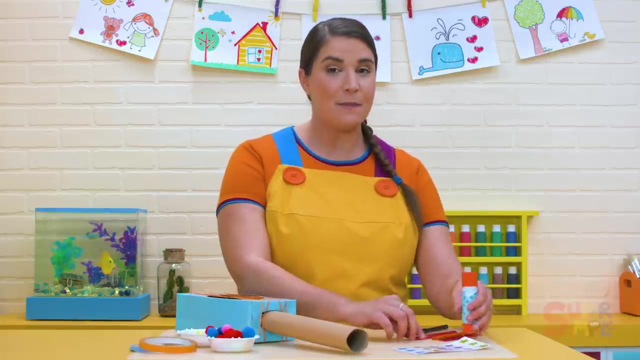 Different elastic bands will make different sounds. You might like to experiment using thin ones or thicker ones, smaller ones or bigger ones. See what sound you like for your guitar. To make our guitar sound a little bit better, we're going to add in some popsicle sticks. 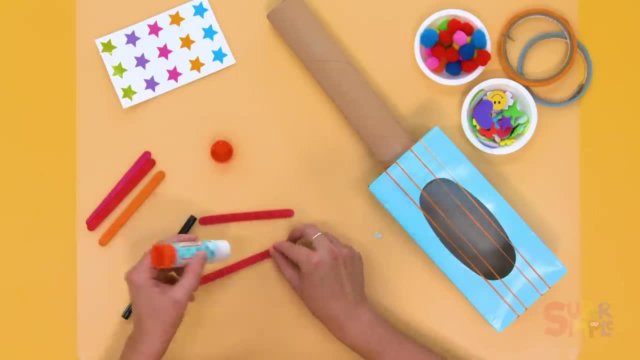 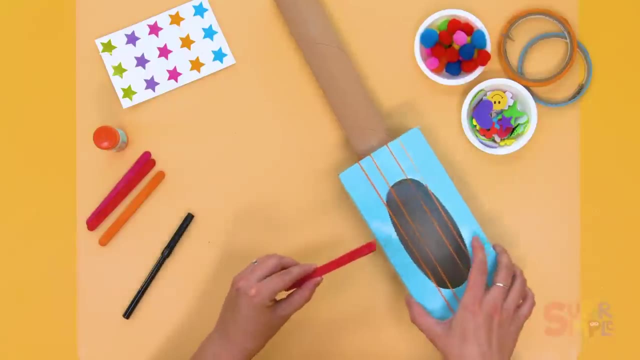 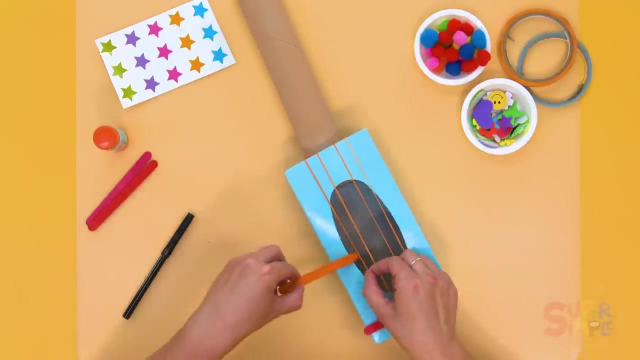 We can glue two regular popsicle sticks on top of each other just to make it a little bit thicker. Here we go. We'll carefully stick them underneath the elastic bands and just push them to one side. I have another one here. Push it to the other side. 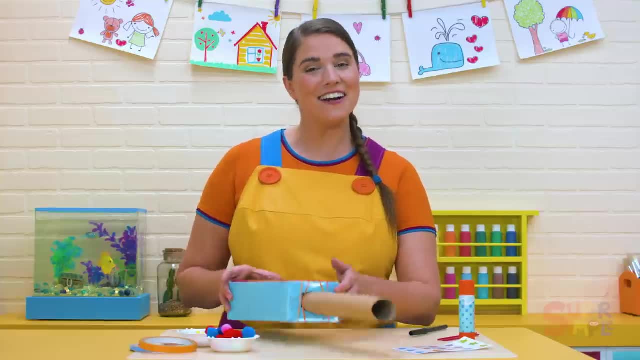 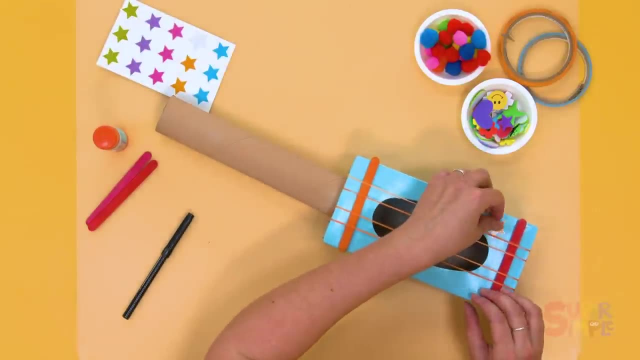 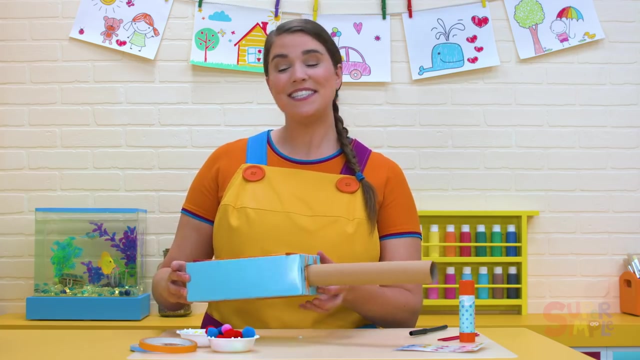 And that'll help make it sound a little bit better. Now our guitar is all ready to decorate. You can decorate yours any way you like, maybe with some stickers, maybe a smiley face sticker. Look at that And once it's all decorated, it might look like this: 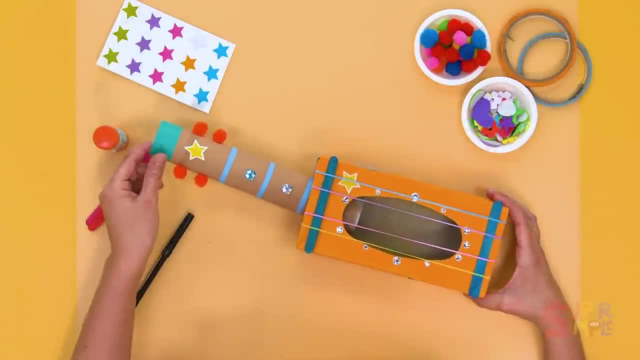 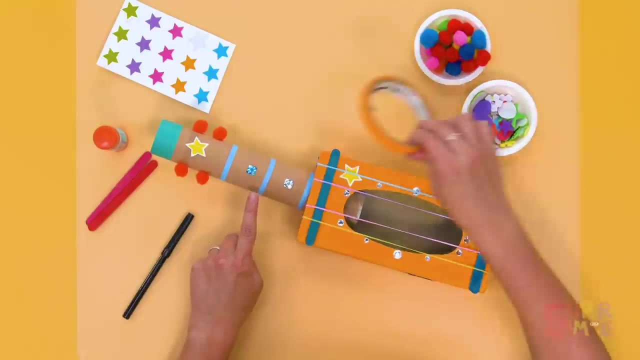 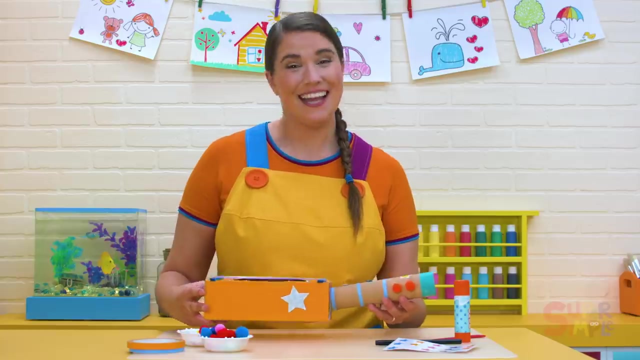 I added in some pom-poms for the knobs on the neck, lots of different stickers and jewels and even some double-sided tape on the neck of the guitar. Just wrapped it around so it looks like a real guitar neck. Look at that. 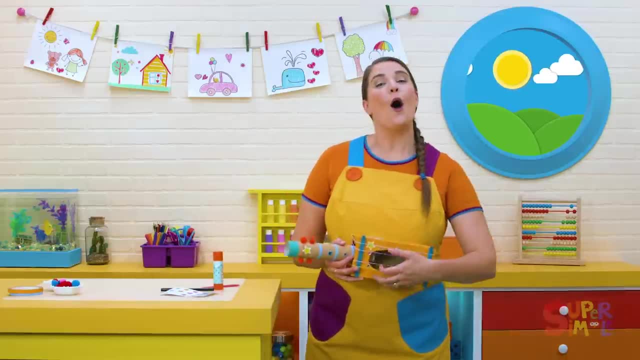 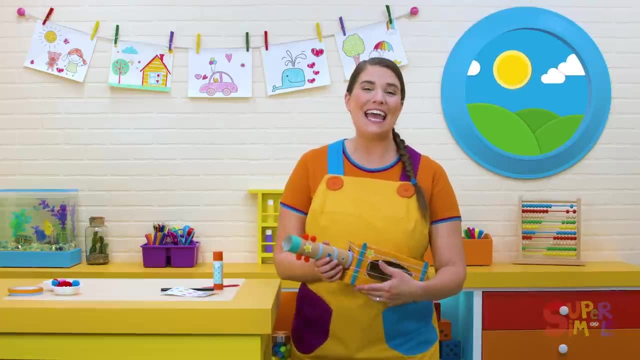 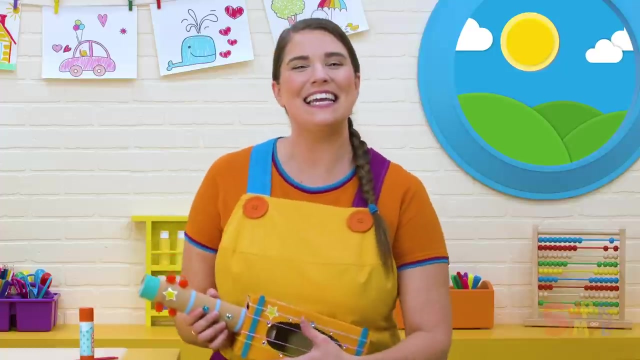 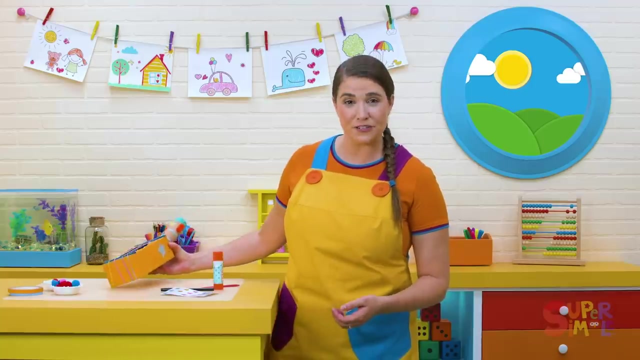 Should we try playing it. Oh, when the guitar comes marching in. Oh, when the guitar comes marching in, It goes. When the guitar comes marching in, Learning a new instrument can be tricky. I remember when I was first learning the guitar it felt very hard to do. 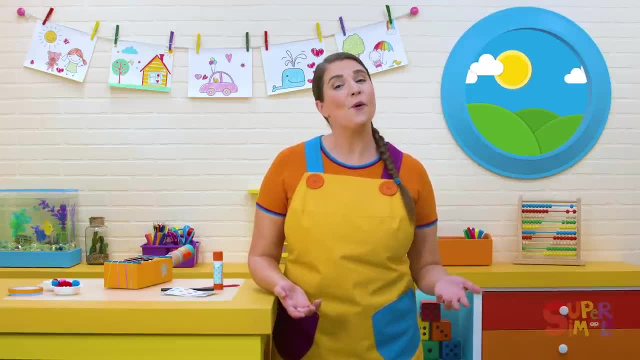 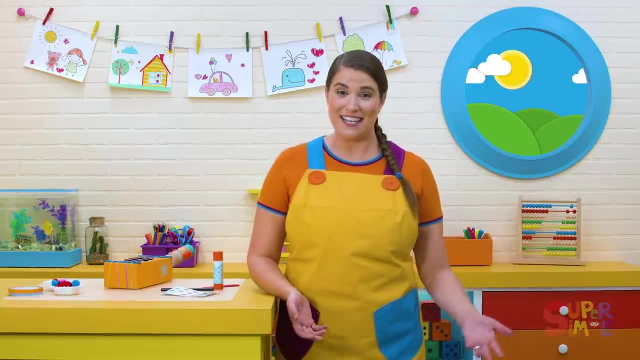 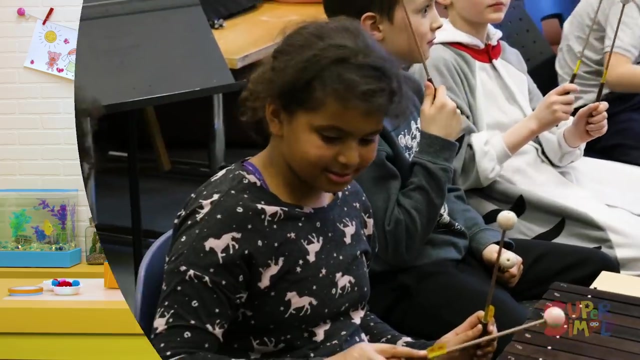 I had to practice a lot. Practice is an important part of learning something new. Let's go on a field trip and we'll meet some young musicians and hear what they have to say about learning a new instrument. Come on, Hi, Hi. 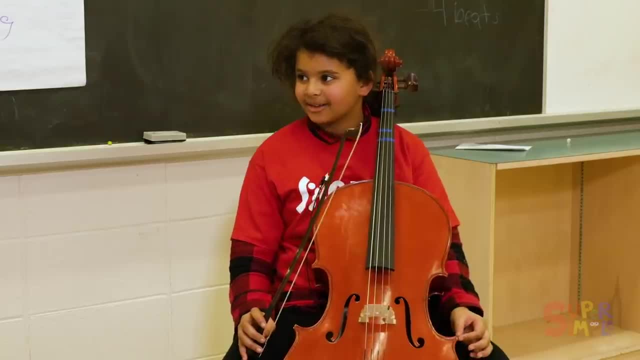 What's your name, Rafi, And what instrument do you play? The cello. The cello is beautiful. It's such a big instrument. Do you like playing the cello? Yes, When you first started playing the cello, what was that like? 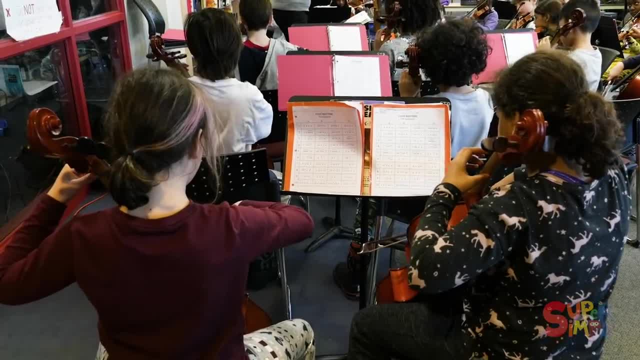 It was hard, but then it got easier. Yeah, I'm sure it's not easy to learn something new right Then. now you really like it. Yes, What do you like most about it? I like the sound and it's also really fun. 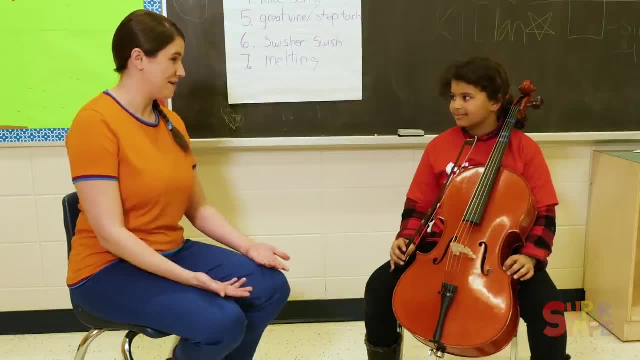 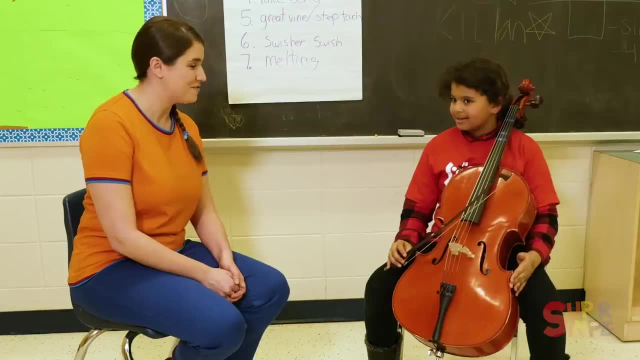 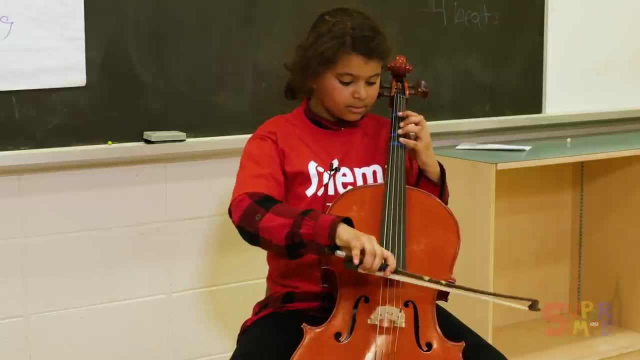 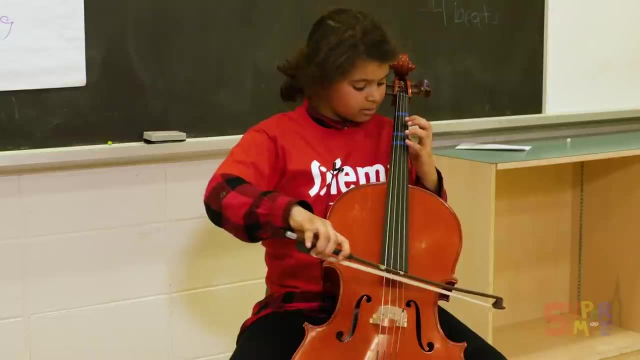 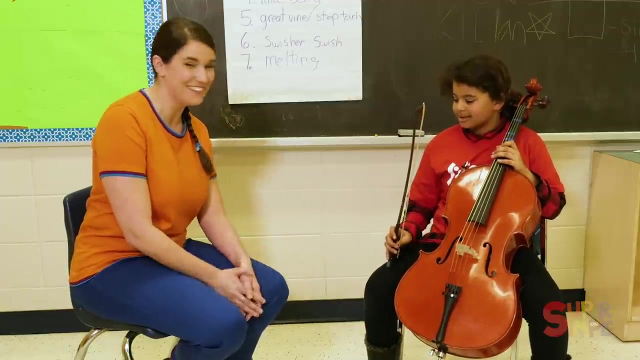 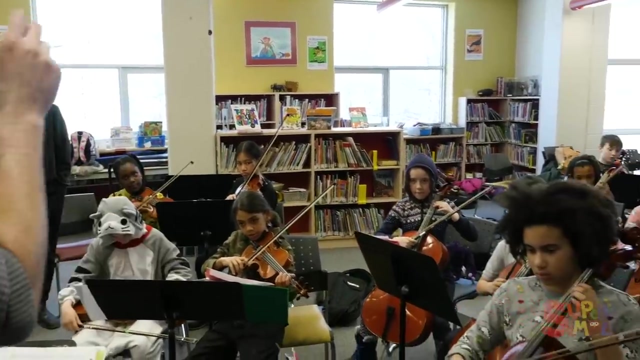 It's not easy to play this. Can you play us something? Sure, That's beautiful. I really like the cello. Thanks, Rafi. 1, 2, 3, 4, 5, 6, 7, 8,, 9,, 10,, 11,, 12,, 13,, 14,, 15,, 18,, 19,, 20,, 21,, 22,, 23,, 24, 25,. 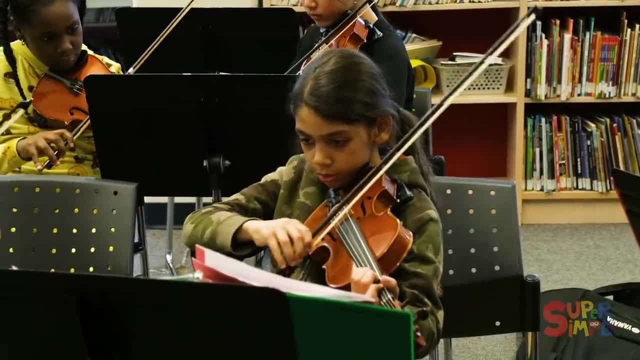 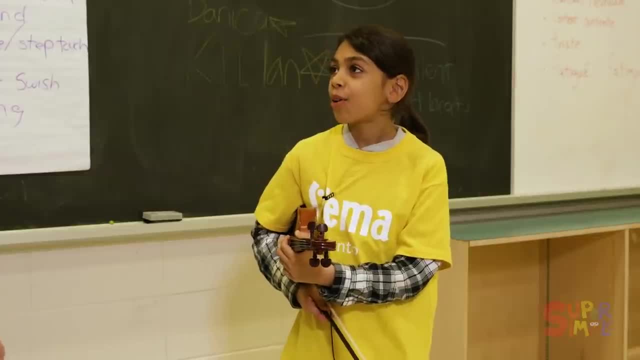 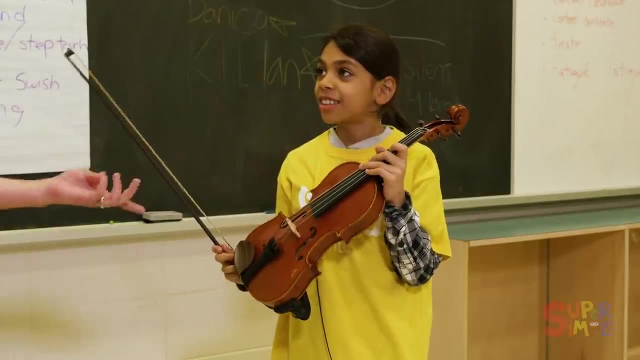 Hi Hi. What's your name? Pao Wan. Hi, Pao Wan, How old are you? Nine, Nine years old. And what instrument do you play? Viola, A viola. It looks a lot like a violin. 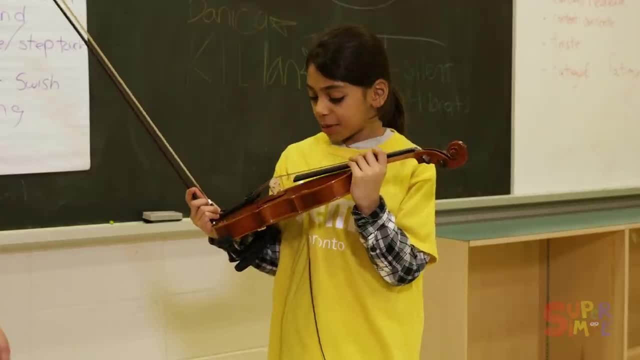 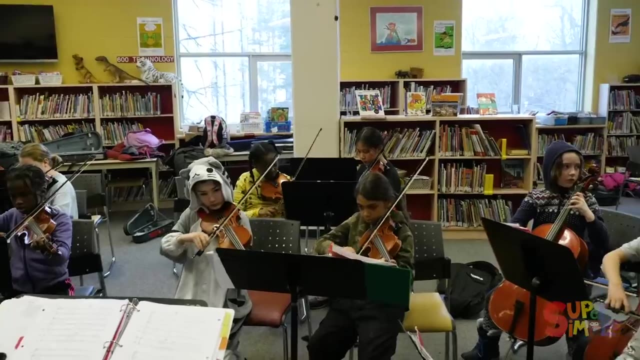 What's the difference between a viola and a violin? It's a little bigger and it has a different string. A little bit bigger than a violin. Nice, How long have you been playing the viola? for One year. So what would you tell somebody who wanted to learn an instrument? 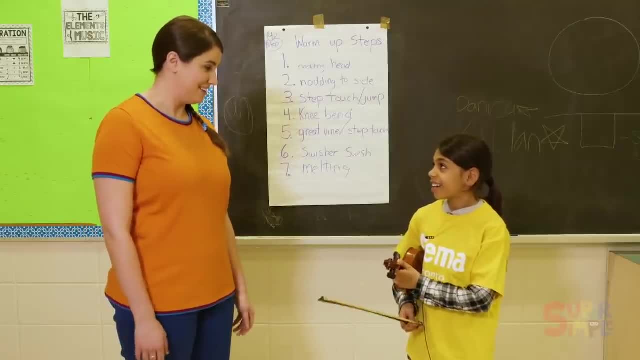 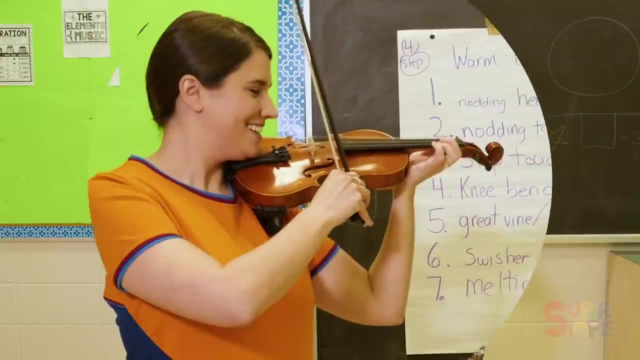 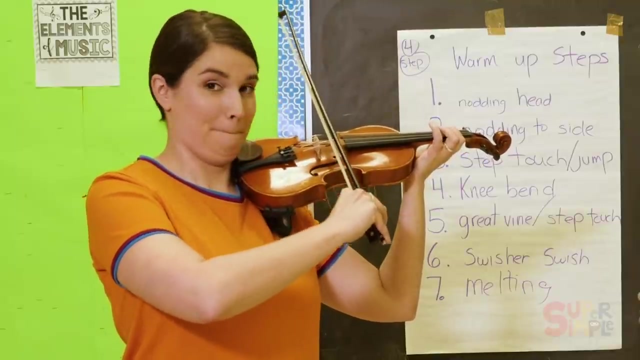 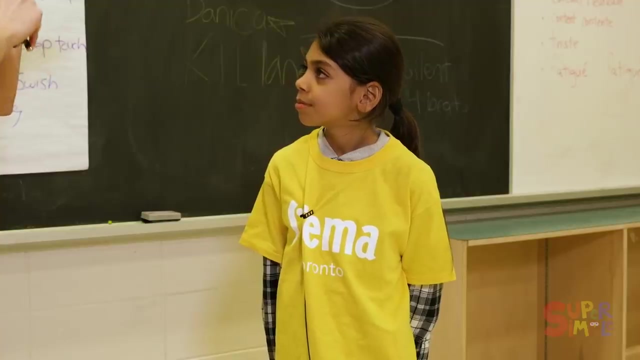 but they've never played one before. Try one, Just try one. Yeah, Yeah, Here You're going to let me play yours. Yeah, What? Thank you so much. That's so nice. Thanks so much for letting me try. 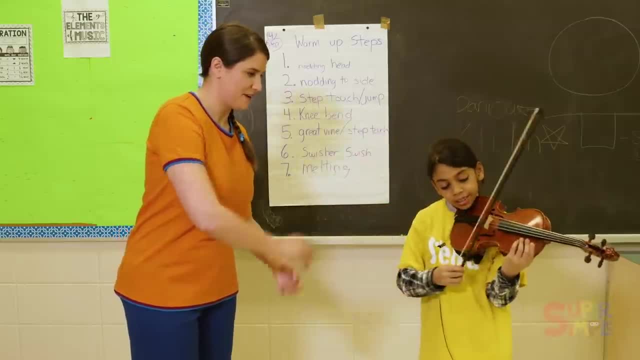 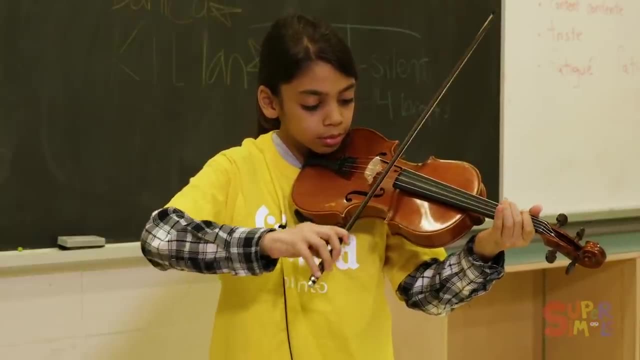 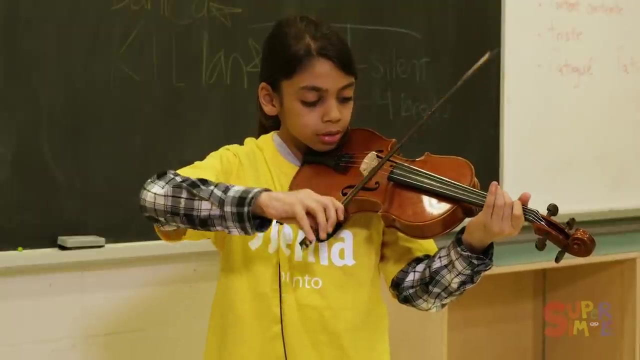 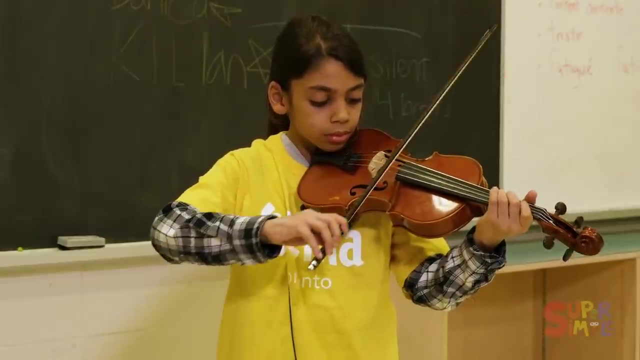 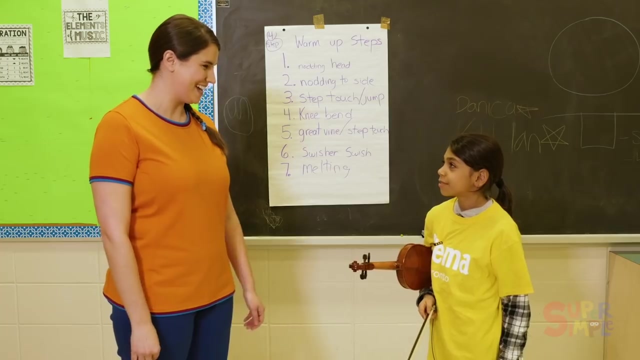 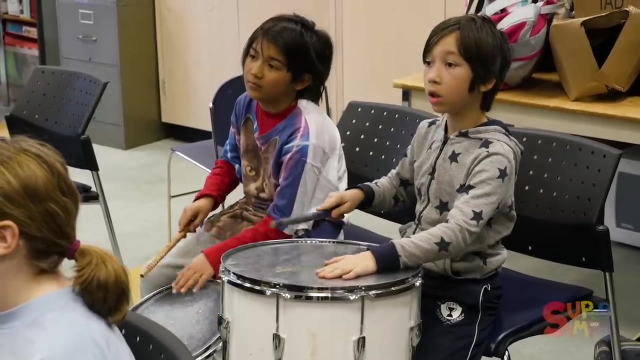 That's really great. Will you play us something? Okay, Yeah, I'm sure you're a lot better. That was amazing, Thank you. Thank you so much for playing that. These students are all learning a new musical instrument with an after school music program called Systema Toronto. 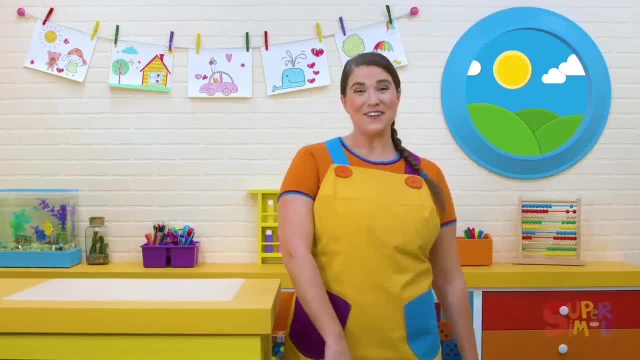 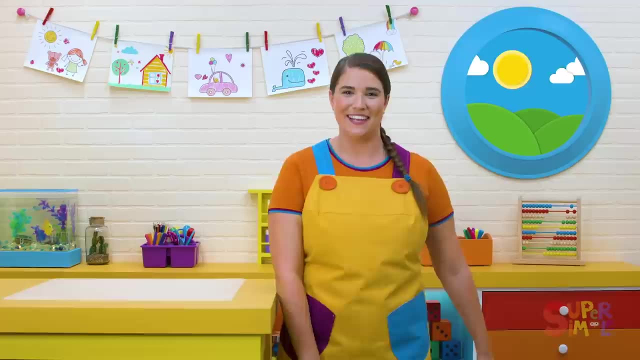 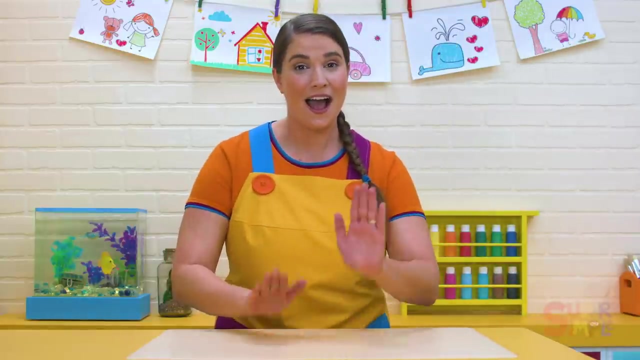 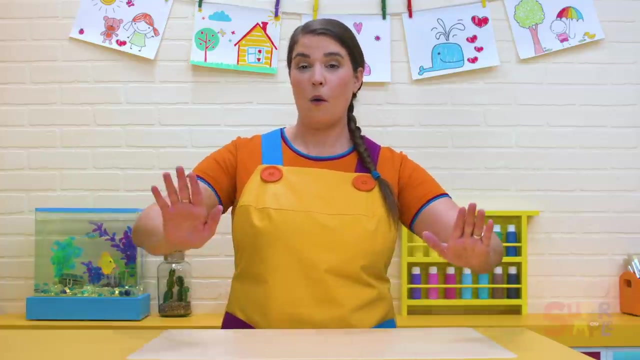 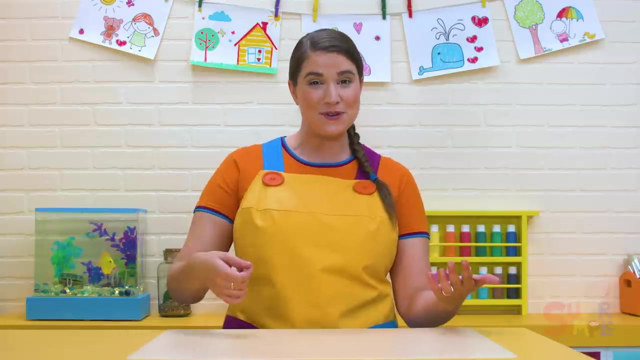 It's amazing. Those are some incredible instruments and musicians. Practicing an instrument can be lots of fun. Let's practice one together. You probably have this instrument At home: a drum. anything can be a drum. You can use a table or your belly, maybe an upside down cooking pot with a wooden spoon, or you might have a toy drum like this. 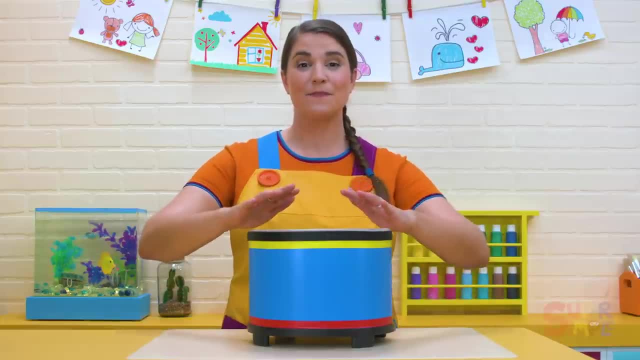 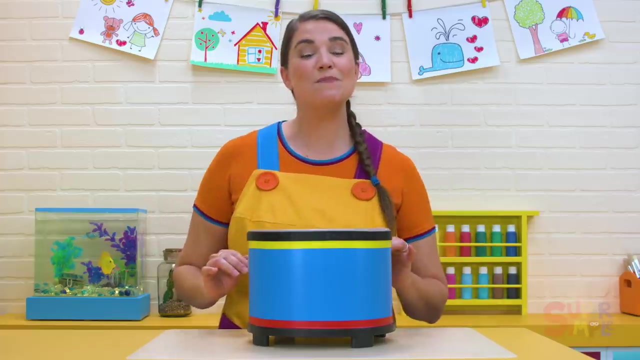 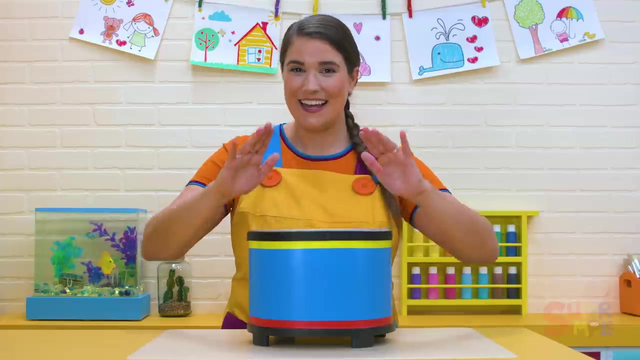 Do you have your drums ready? Let's practice. Can you try that? Your turn? Very nice, Try this. Now you go. That's it. Let's play all together. We'll start slow, then go faster. Nice and slow. 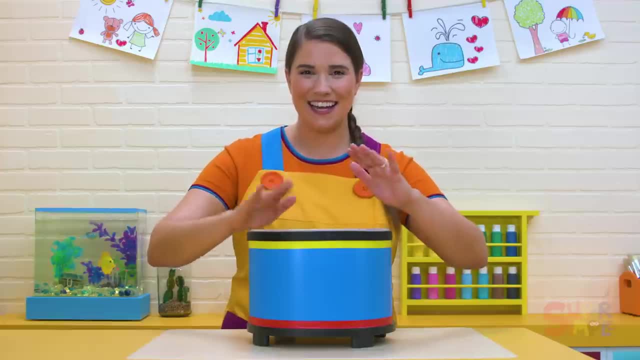 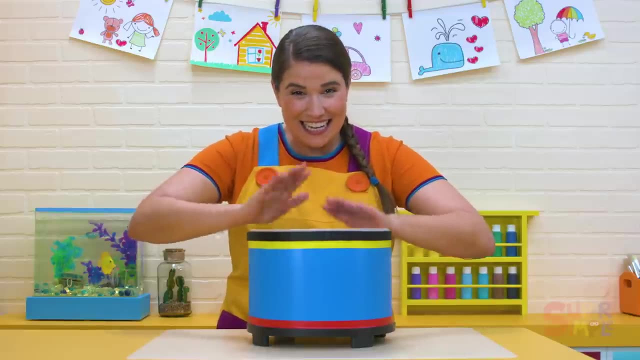 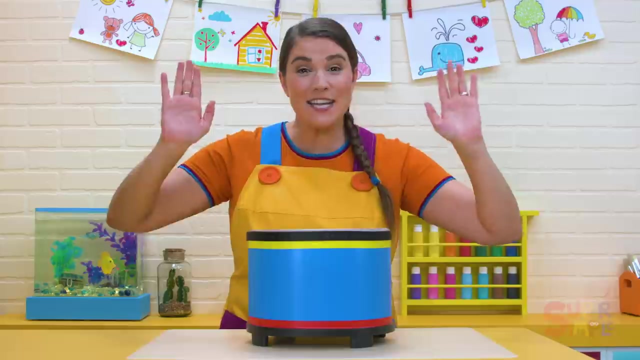 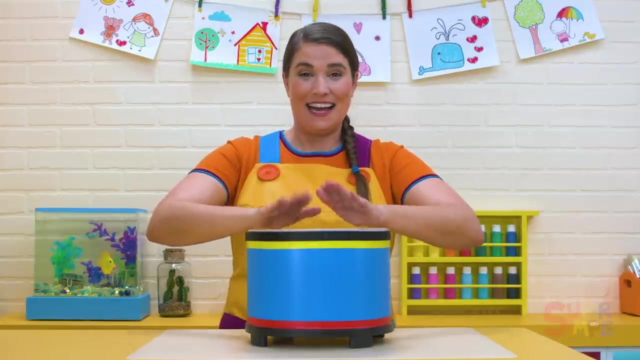 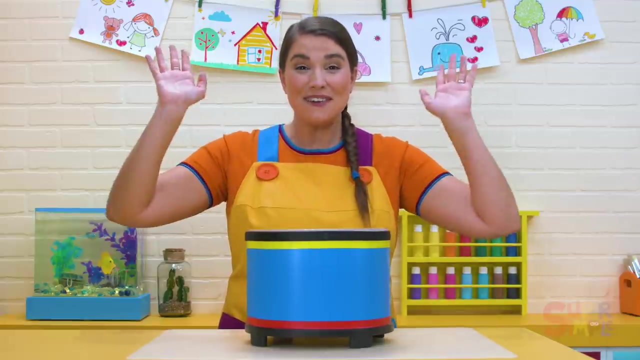 A little faster, Faster, Faster. Let's go really fast And stop, Don't move. Let's go And stop, Go, Stop, Go, Stop, Go, Stop, Nice drum, Nice drum, Drum, practicing everybody.